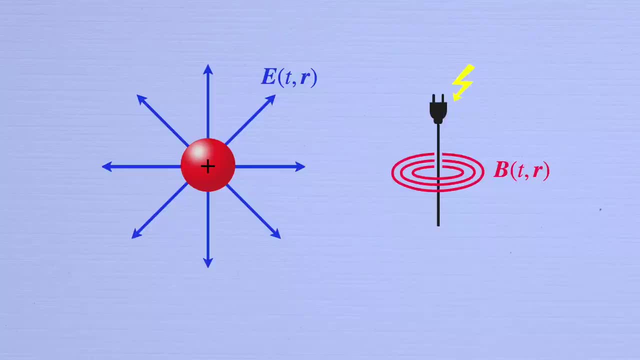 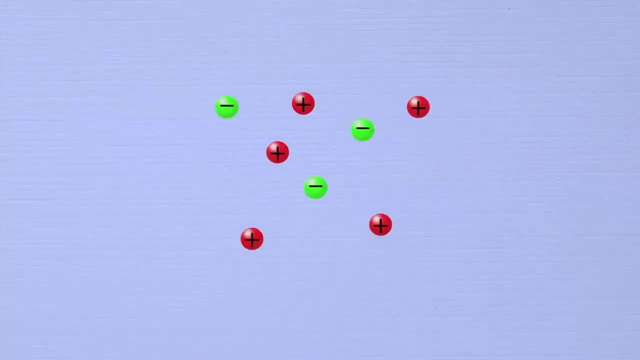 your eyeballs at this very moment. In a field theory like electromagnetism, the connection between symmetries and conservation laws becomes even deeper. You're no doubt familiar with the conservation of electric charge, for example, But the conservation of charge isn't simply the statement that the total amount of electric charge in the universe 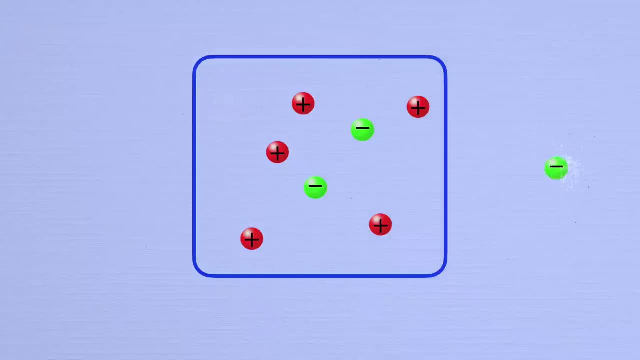 is a constant. For example, if an electron disappeared in Tokyo at the same moment a muon appeared next to Tau Ceti, the total amount of charge would not have changed. But a conservation law in field theory is stronger than that. Charge is conserved locally, meaning that the only way 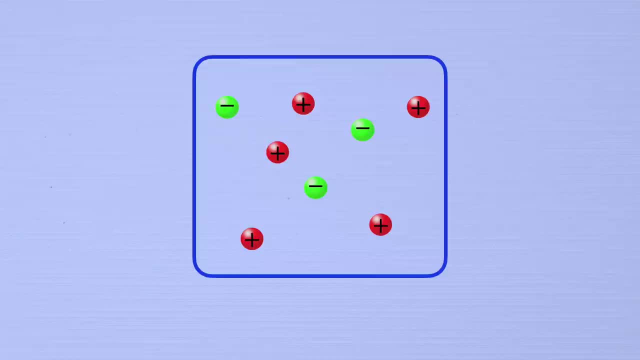 the amount of charge can change inside any box, large or small is if a current continuously carries charges in it. But if conservation laws result from symmetries of nature, then what symmetry is responsible for the conservation of electric charge? We'll discover the answer in this video. 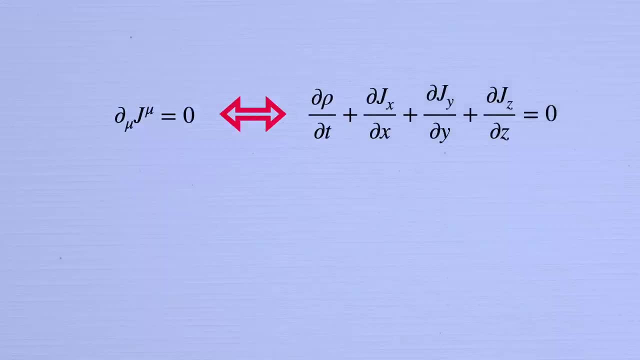 In the first part we'll see how local conservation laws arise in field theory and how they're captured by the continuity equation which constrains the charge density rho and the current density j. Then, in the second part, we'll identify the associated symmetry. 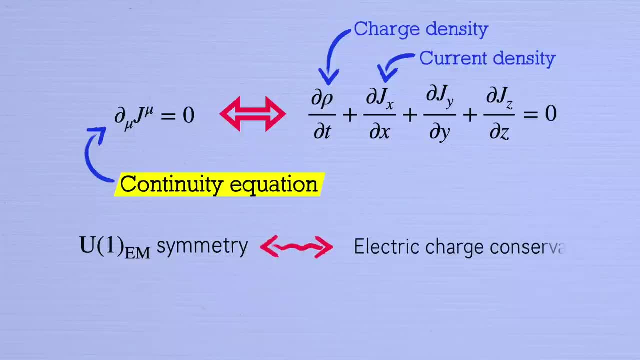 known as U1, in a theory like electromagnetism that's tied to the conservation of electric charge by Noether's theorem, And in part three we'll put the pieces together and write down the simplest example of a gauge theory. By the way, I should point out that the U1 of electromagnetism is not literally the U1 in the 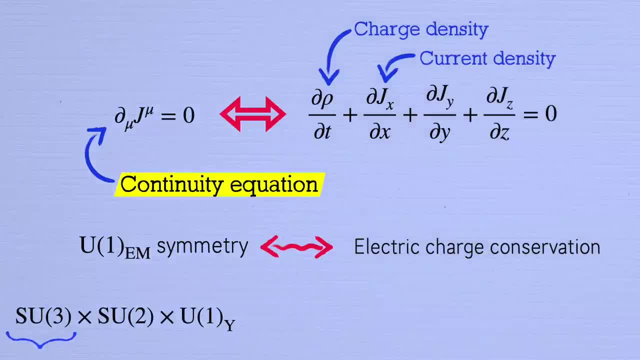 symmetry that labels the standard model. The SU3 factor stands for the theory of the strong force, the SU2 stands for the weak force and the third U1 is called hypercharge. The electromagnetic force is a different but related U1 that sits inside here. 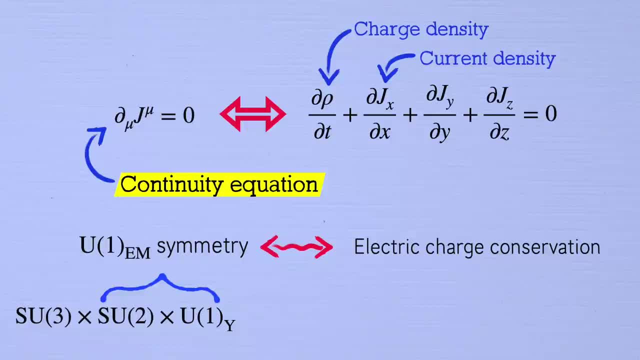 and electromagnetism falls out, after the famous Higgs field does its work. We'll see how that works in the next part. We'll see how that works in the next part. We'll see how that works in the next part. We'll better understand what all these symbols mean as we go along though the Higgs mechanism. 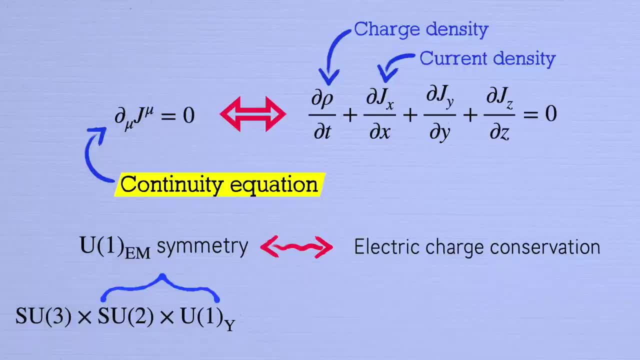 will have to wait for another video. Let me know in the comments if that's something you'd be interested in. We're getting into an advanced subject here, so this lesson isn't going to be easy, But considering we're talking about some of the deepest principles of nature. 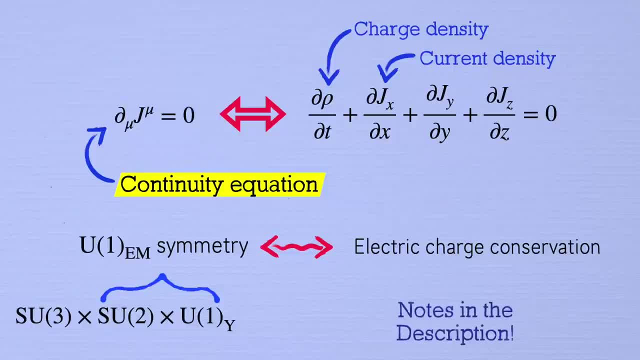 it's definitely going to be worth the effort to understand- And, as always, you can get the notes that I've written at the link in the description to take your time understanding all of these ideas. Before we get too deep into the physics, though, 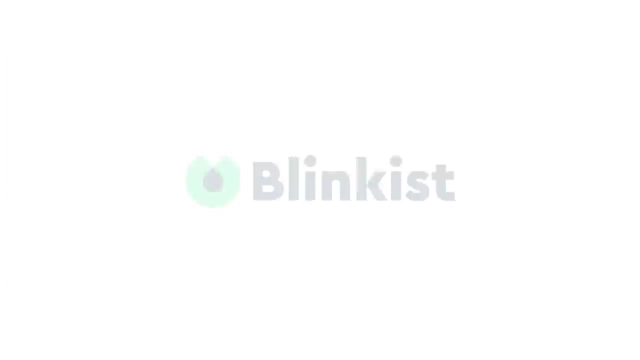 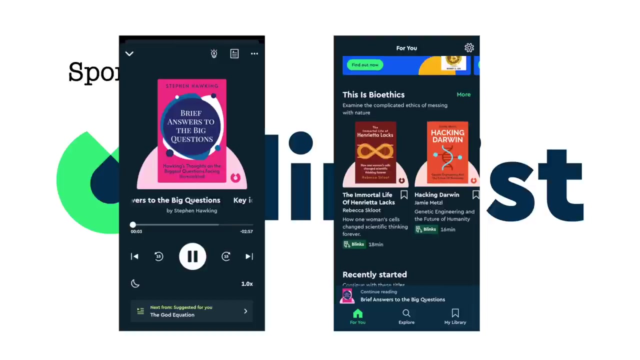 let me take a quick second to tell you about this video's sponsor, Blinkist. Blinkist is a really cool app that lets you take away the key insights from a huge library of non-fiction books with bite-sized 15-minute summaries that you can listen to or read whenever you want, And they even cover. 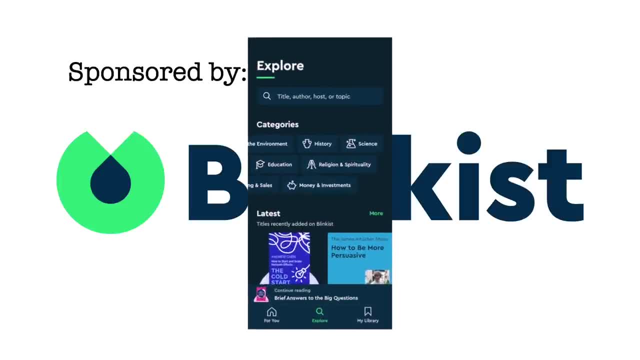 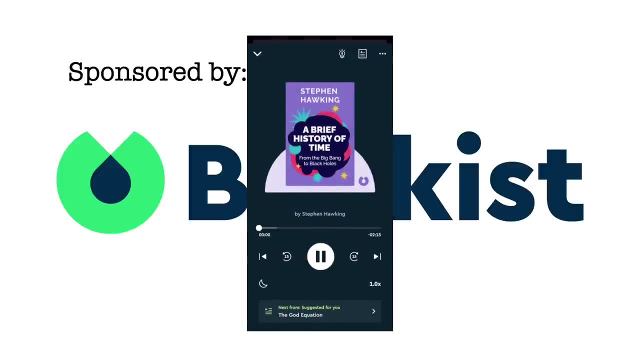 a lot of podcasts too, So of course I had to go in and first check out the science book selection. There's some classics, of course, like A Brief History of Time by Stephen Hawking, which is a whirlwind tour of physics from gravity and relativity to quantum mechanics. 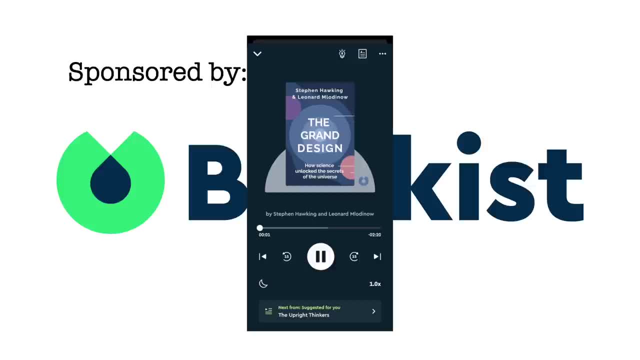 and the arrow of time, And also his book with Leonard Mlodinow, The Grand Design, which is an exploration of how science has transformed the way we look at the world, And Hawking's last book, Brief Answers to the Big Questions, which is about his thoughts about 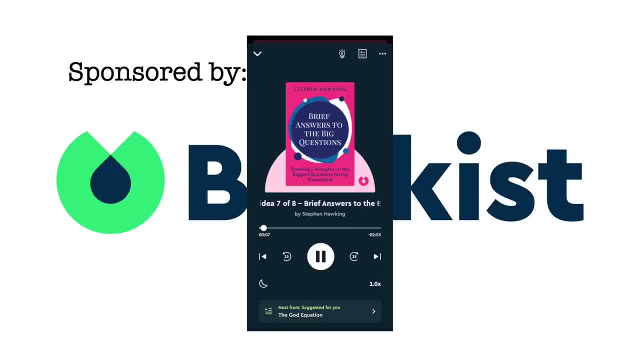 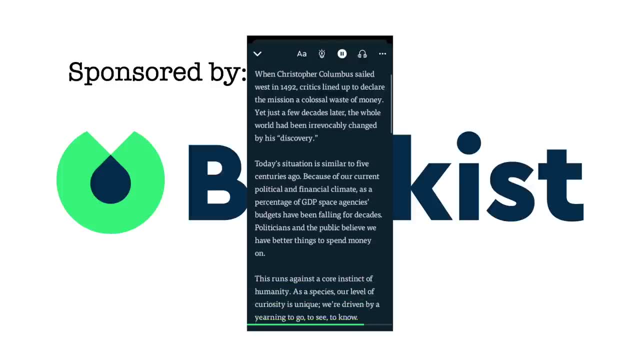 where the universe came from and where we as a species are going. Hawking was working on it right up until he passed away in 2018.. One key thing he argues for is how important it is that we begin to expand beyond Earth. He thinks that it's within reach to set up a moon base or send. 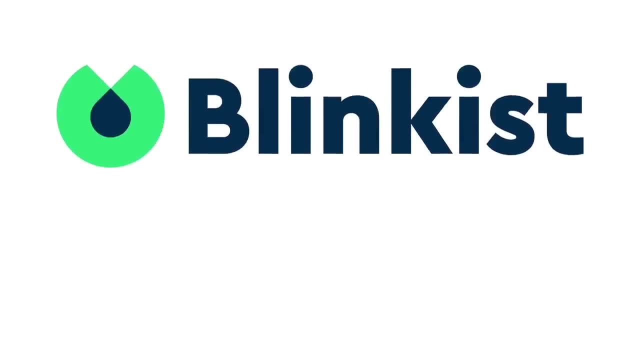 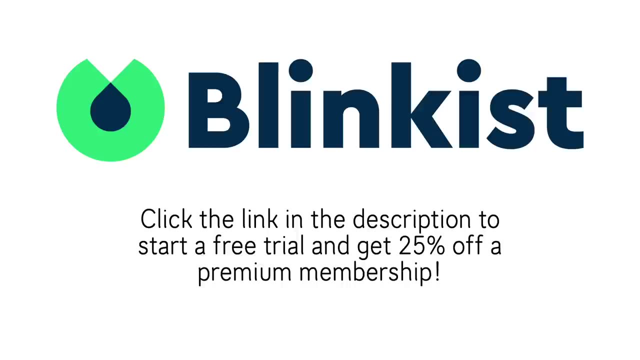 a manned mission to Mars in the next 50 years. Right now, if you use the link that I've shared down in the description, you can start a free 7-day trial of Blinkist and then get 25% off a premium membership if you decide to sign up. So go try it out. it's a really nice app that. 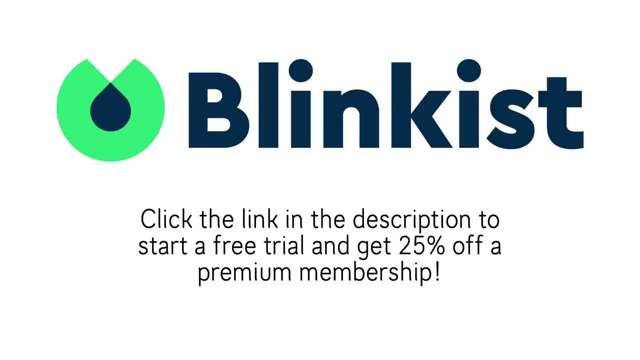 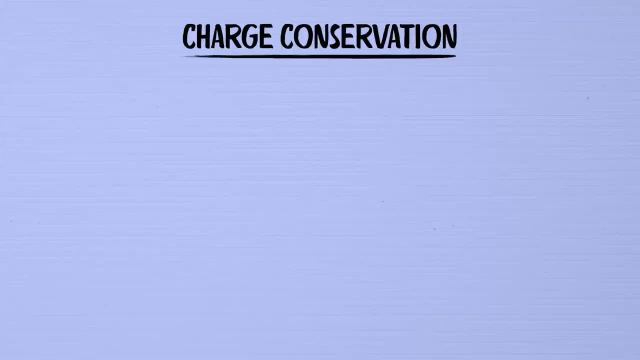 lets you understand and grow from big ideas in 15 minutes, And thank you so much to Blinkist for sponsoring this video. The first thing we need to do to understand the U1 symmetry of the standard model is to sort out what it means for electric charge to be locally conserved, which you may or 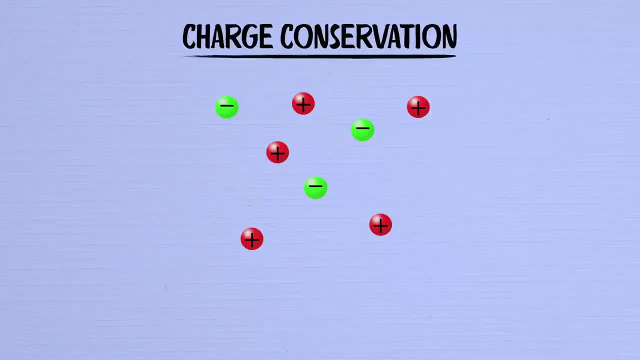 may not have learned about before in a class on E&M. This is going to be essential for understanding how conservation laws emerge from symmetries in field theory, so it's important to take a few minutes to get it straight. Say: we have some region of space v To measure the amount of charge inside the box. 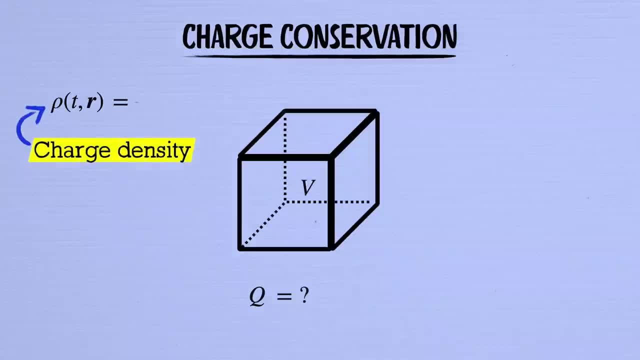 we start from the charge density rho, which represents the amount of charge per volume at any point in the box at any time. t. In other words, if we look at any infinitesimally tiny box, the amount of charge inside it is its little volume dxdydz times the charge per volume rho. 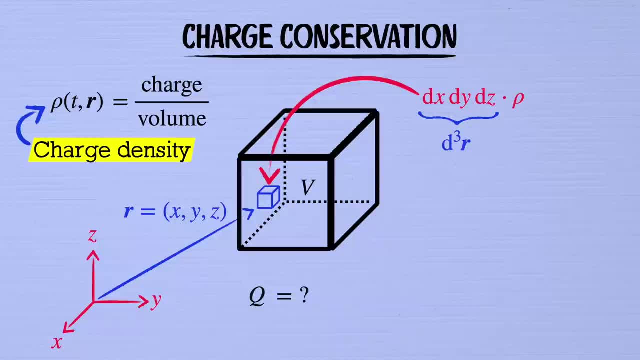 I'll write that volume as d3r for short To find the total charge inside our whole box. we just dice it up into lots of little pieces like this and then we add them all up by integrating over the region. This is the total amount of charge q in our big box. v at any time, t. 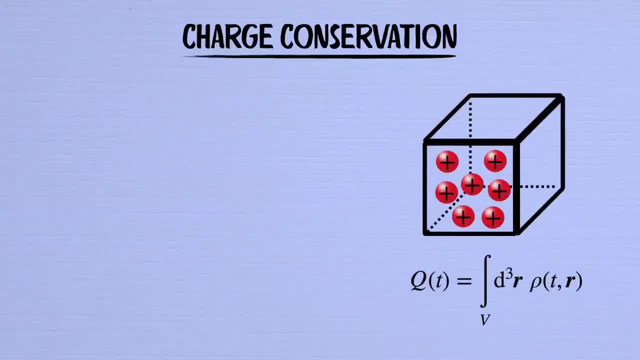 What charge conservation means is that the only way q can change with time is if some of the charges inside the box move outside through the surface or if additional charged particles from outside make their way in. These moving charges would constitute an electric current, the amount of charge per second leaving through the surface of the box. Let's call that. 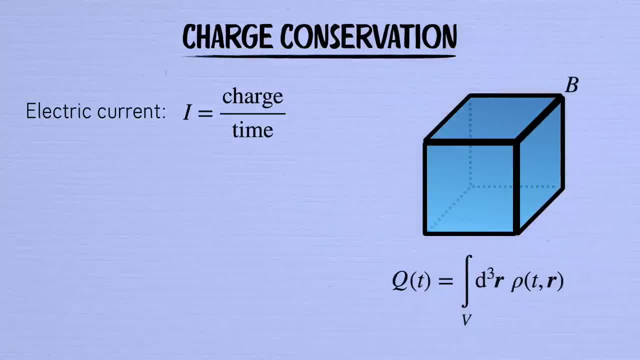 boundary surface b, Then what we need to know is, given some current, how much charge is flowing through this boundary b at any moment? Similar to rho, which measured the charge density per volume of space, we measure the amount of current by the current density j. But there are some. 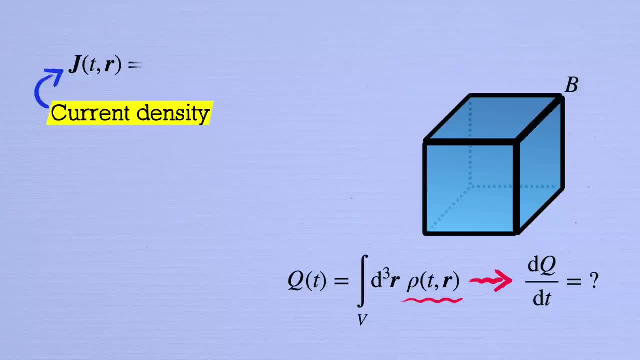 important differences between rho and j. Note first of all that j is a vector with components jx, jy and jz, because a current can flow in any direction in space. Also, whereas rho was the amount of charge per unit volume which we used to find the total charge density, 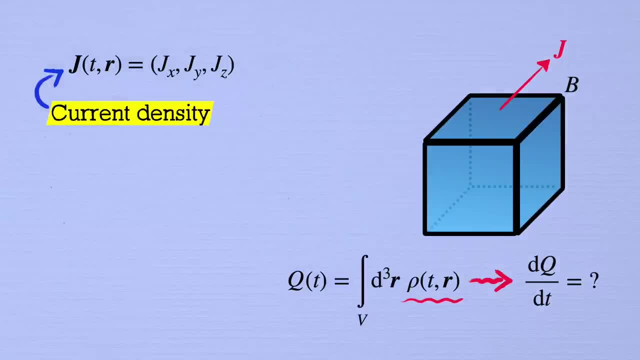 the total amount of charge inside the box. with j, we want to find the amount of current flowing out through the boundary surface. We therefore define j to be the current per unit area rather than per unit volume. Let's look at the top surface of our box, for example. 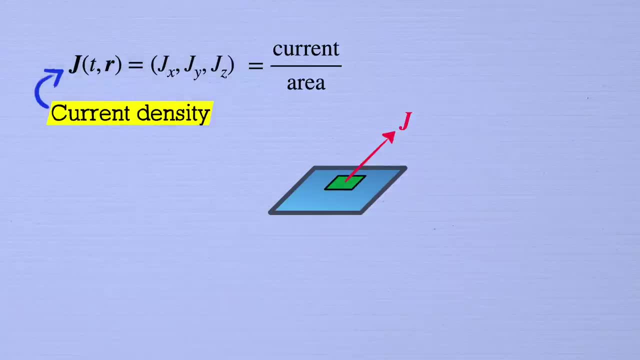 Take a little patch of the surface of width dx and length dy, Since we want to know how much current is flowing out of the box. what we care about in this case is the z component of j. at that point jx and jy just measure the current flowing parallel to the surface, Then the amount. 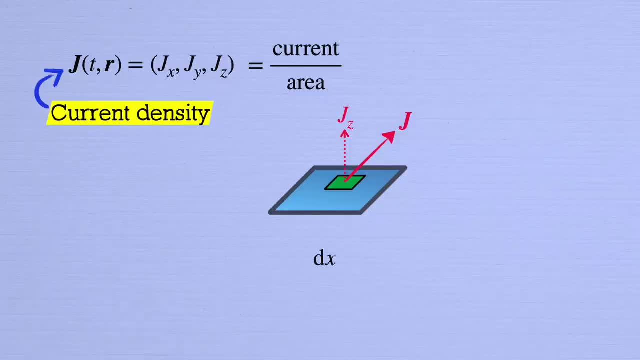 of current passing through. that little patch is given by its area dx dy times jz, the current per area in the z direction. We get the total current passing through the whole top surface by integrating over it At any instant in time. this is the amount of charge per second leaving. 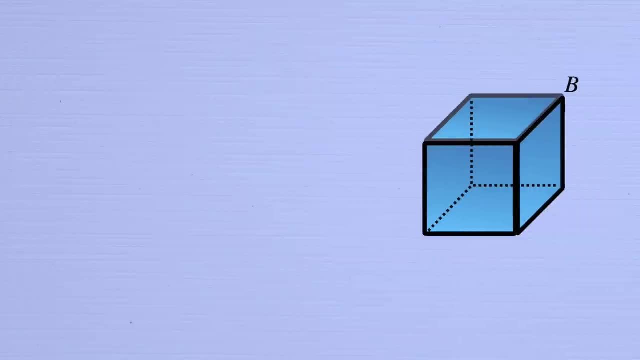 through the top surface of the box, Of course. now we need to do the same to find the current passing through the other sides of the box and then add them all up to get the total current going out through the surface And in general our volume v needn't be a neat. 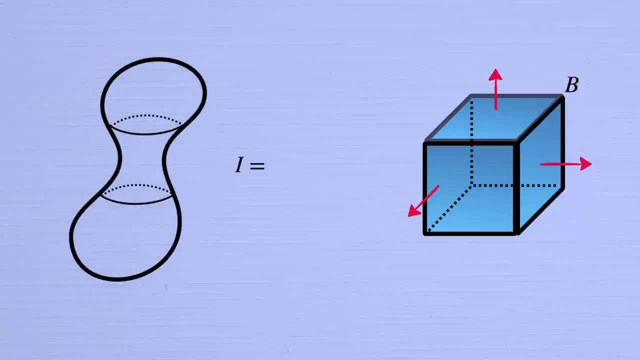 box, and its boundary needn't be a cubical surface. It could be some misshapen blob instead. But the idea is the same. We slice up the surface into many little patches, each of area da. Then we multiply that by the current per area flowing out through the patch. 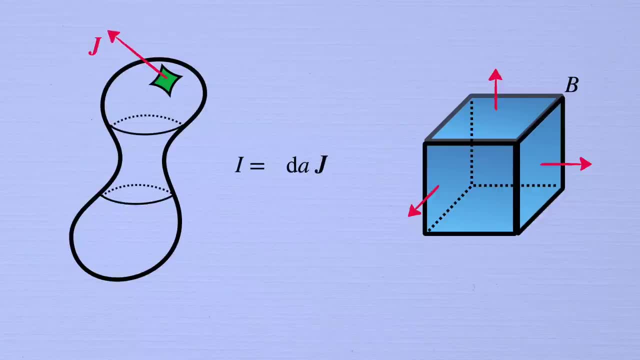 That's given by j at that point. But again, we need to pick out the component that points perpendicular to the surface in order to obtain the amount of current going out. We can do that by finding the unit vector n hat that's perpendicular to the surface at that point. 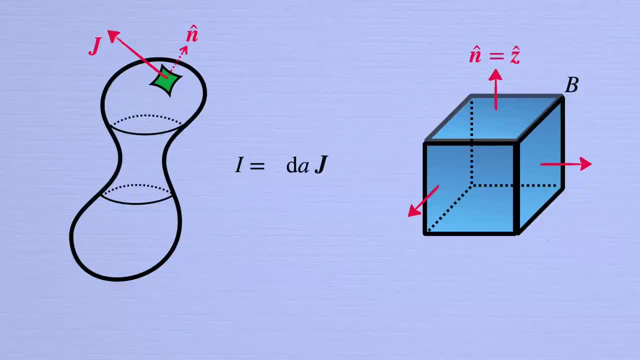 For example, on the top surface of the box n hat equals z hat was the unit vector pointing up in the z direction. On the right surface it would be y hat pointing to the right in the y direction, and so on. Then we can pick out the perpendicular component of j by taking the dot product. 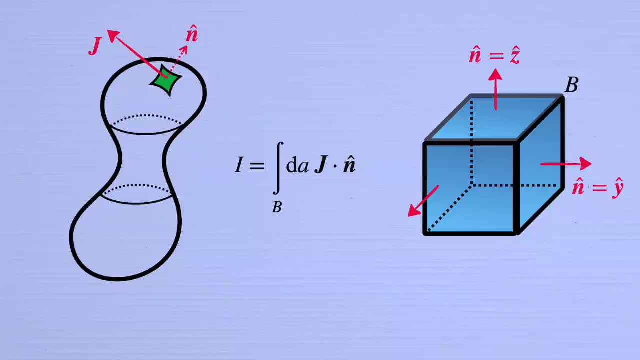 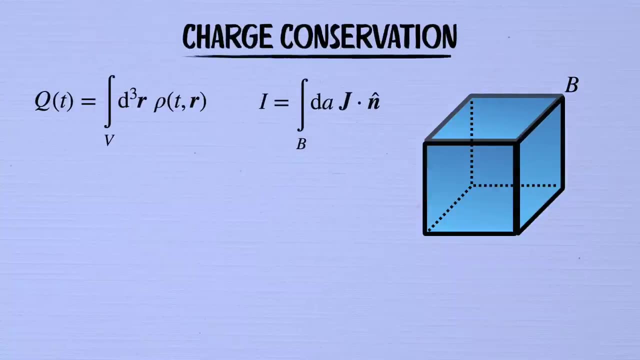 j, dot n. Finally, we add it all up by integrating over the surface And that gives us the total amount of charge, leaving the volume per second, Which brings us back to charge conservation. Local conservation of charge is the statement that if charge i per unit time flows out through the boundary surface, then the amount of charge inside the 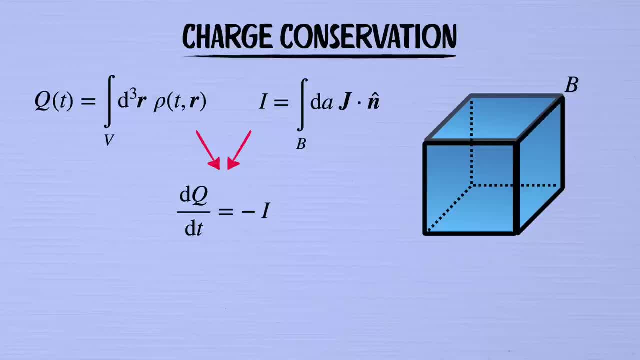 volume of the box goes down at that same rate. dq by dt equals minus i. This is the mathematical statement of charge conservation. Again, the minus sign is there because we defined positive i to mean that current is flowing out through the boundary, in which case the amount of charge inside the box is decreasing at that same rate. 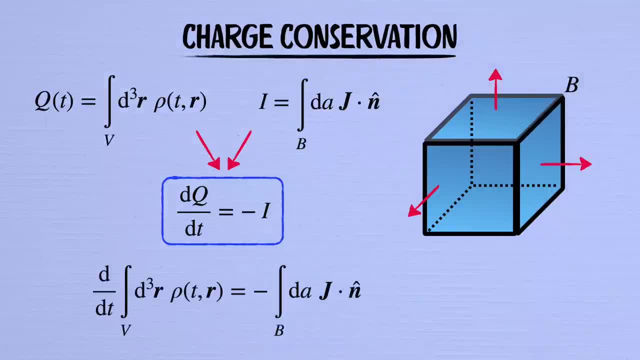 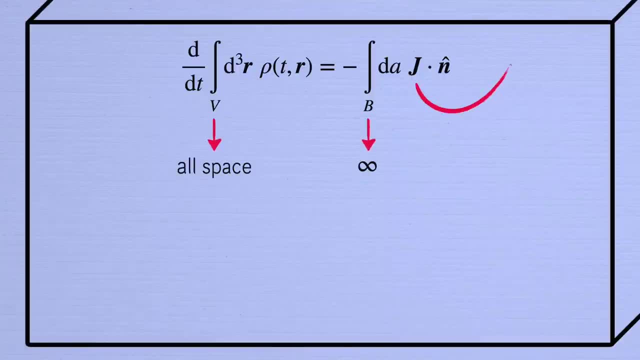 Failed out the charge conservation equation looks like this: If, in particular, we took v to encompass all of space so that the boundary b is going to infinity, the current density had better go to zero there in any physically reasonable setup, since there's nowhere left. 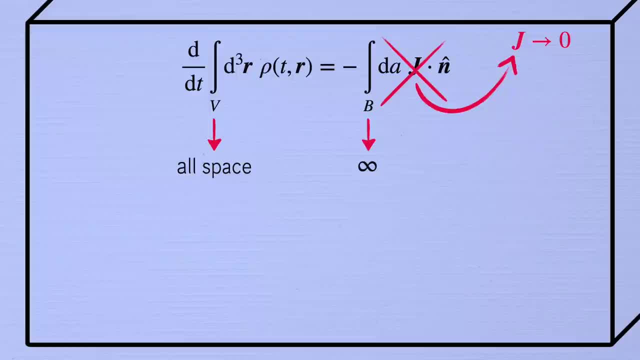 for the current to flow out to. Then the right hand side vanishes and this equation says that the total charge in all of space is a constant. That's the statement of global charge conservation. But again, local conservation of charge is a stronger statement. 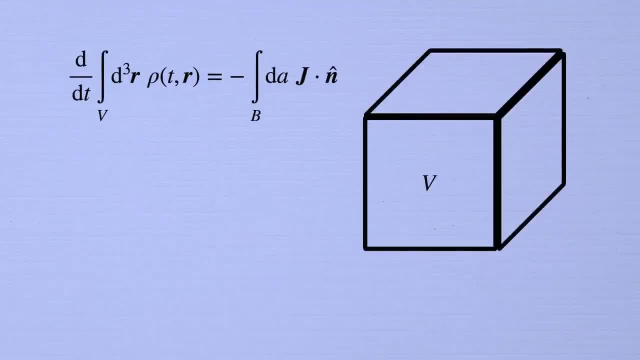 that this equation must hold for any volume v that we like. That's why a charge can't disappear from Tokyo and reappear at Tau Ceti. Instead of choosing v to fill all of space, just build a box around Tokyo. The total charge inside can only change if a current continuously carries charge. 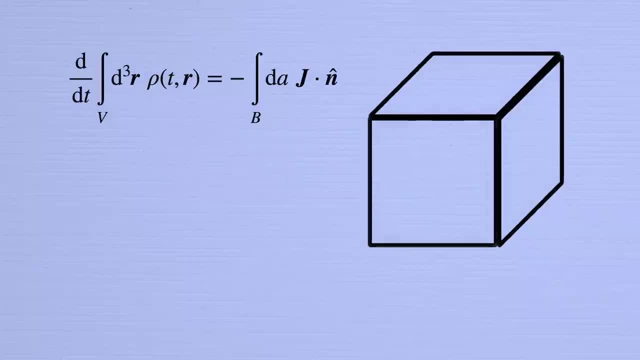 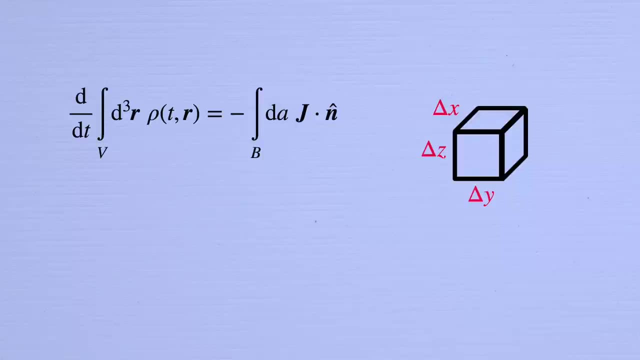 in or out through the surface. On the flip side, we can alternatively take our box to be an infinitesimally small cube whose dimensions- delta x, delta y and delta z- are going to zero. That lets us turn this integral equation into a differential equation, And that's the continuity. 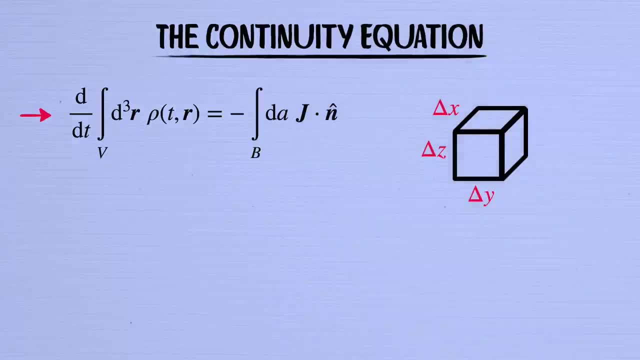 equation that I mentioned at the beginning, which will play an essential role in the equation. Let's first of all bring the d by dt inside the integral on the left. The only change is that it turns into a partial derivative, because rho is a function of both time and space. Now, when we 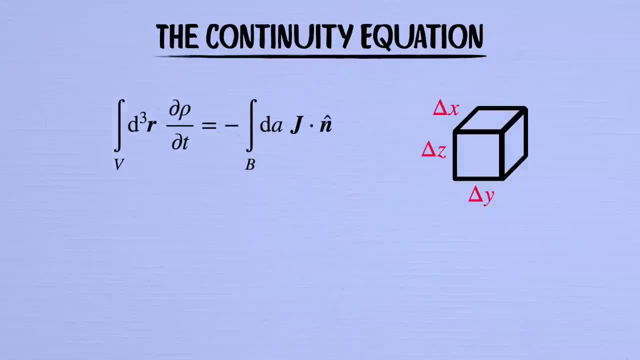 shrink our volume down to a teeny tiny cube, these integrals become pretty boring. On the left, we just get d rho by dt times the volume of the box- delta x, delta y, delta z, The reason being that d rho by dt is essentially constant over this infinitesimally small region. 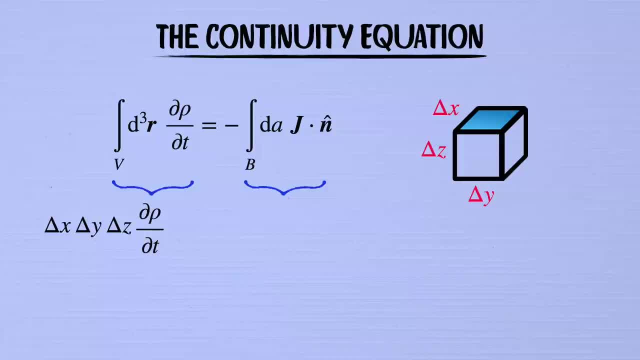 Right hand side is slightly more interesting. Take the top surface again, for example. The outward pointing perpendicular direction is going up, So we get j dot n equals j z evaluated at the top of the box And the area is delta x, delta y. So the top surface contributes delta x, delta y. 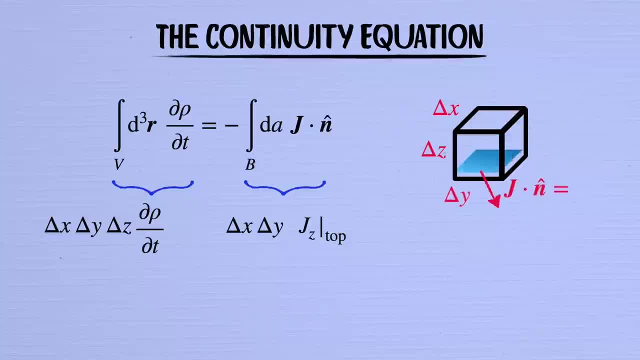 times j z at the top to the integral. For the bottom surface, on the other hand, the outward direction is pointing down. So for that piece of the integral we get j dot. n equals minus j z. Together we're going to get delta x, delta y. 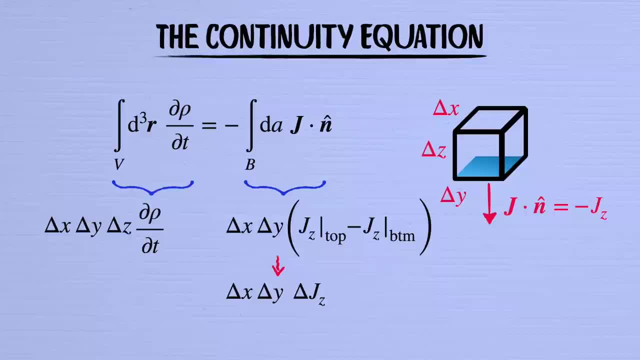 times the change in j z between the top and bottom of the box. We had a factor of the volume on the left hand side of our equation that we're going to want to cancel out. So let me go ahead and multiply by delta z over delta z on the right. Then we 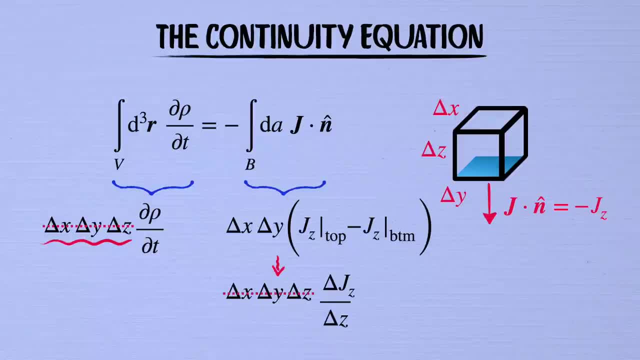 can cross out these common factors and in the limit that the box becomes infinitesimal, we just get the derivative of j z with respect to z. Of course we also have to include the front and back and the right and left surfaces of the box as well. Those give us the derivatives of j- x. 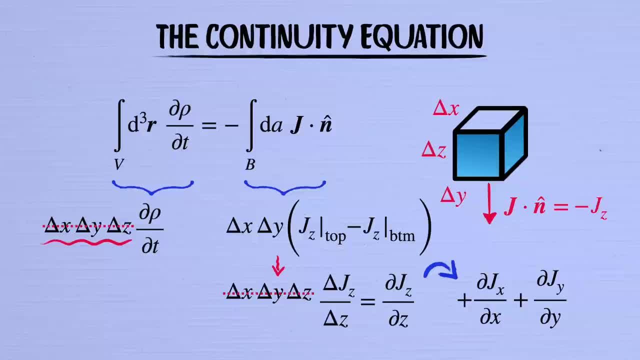 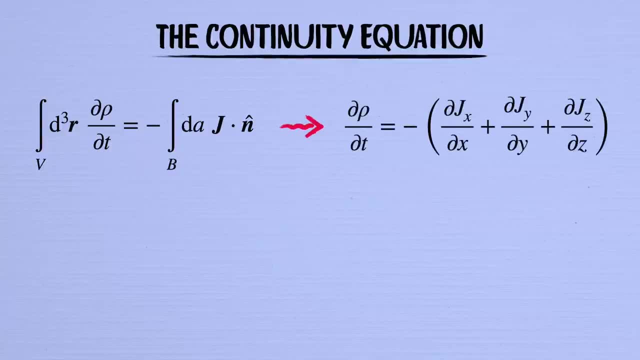 in the x direction and j? y in the y direction. So we get the derivative of j, z with respect to z. All together, our charge conservation equation, when we shrink the region down to be infinitesimally small, becomes d? rho by dt equals minus dxjx plus dyjy plus dzjz. This is the continuity equation. 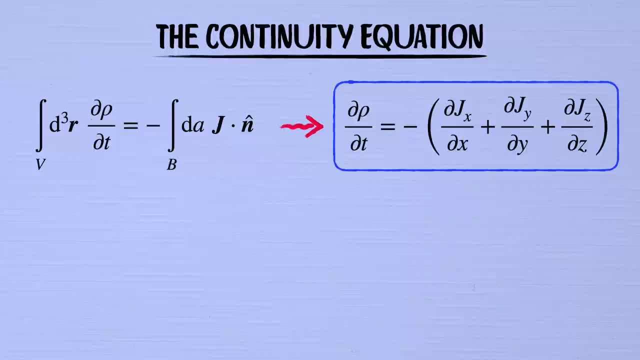 It's the most direct local statement of electric charge conservation and it's the prototype for what it means to have a conservation law in any field theory. We usually shorten it by defining a three-component object called del, with the x, y and z derivatives Denoted by this upside-down. 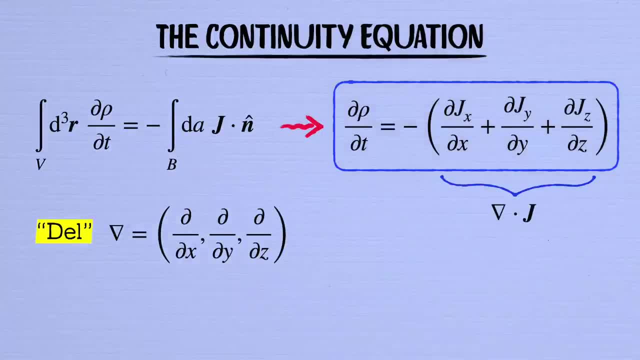 triangle, Then this sum of derivatives is just the dot product of del and j, and we can express the continuity equation more compactly at d rho: by dt plus del dot j equals zero. What we're going to discover is that a local conservation law like this falls out anytime we have a continuous 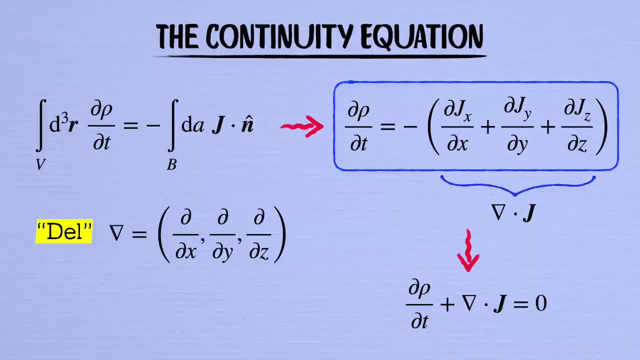 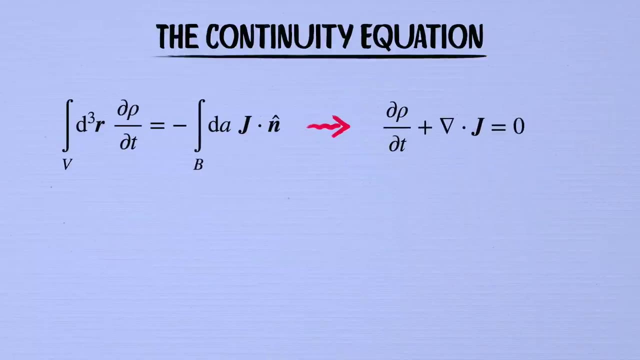 symmetry of a field theory, And this relationship is instrumental to our understanding of particle physics. The symmetry leads to a conservation law, and those charge and current densities become the sources for the fields, just like electric charges and currents produce electric and magnetic fields. By the way, what we basically did in our argument here was discover. 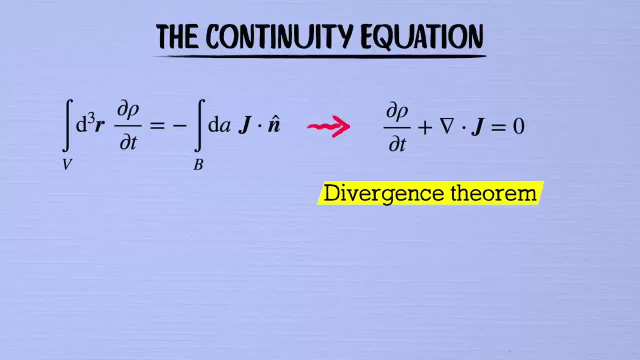 the divergence theorem which you'll learn about in your math classes and which lets us turn an integral over a boundary surface like this into the integral of the derivatives of j over the volume v. inside It's called the divergence theorem because del dot j is called the divergence of j. 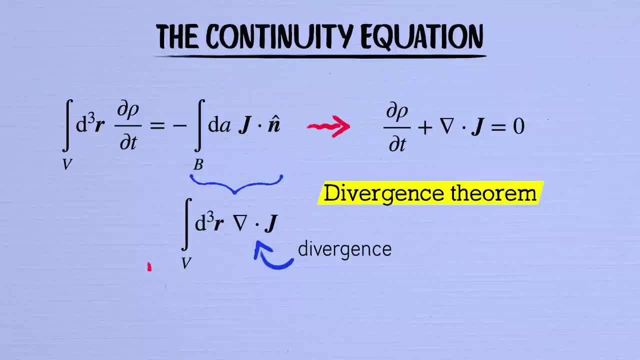 Since our volume v was arbitrary, we can shrink it down and conclude that the integrands d rho by dt and minus del dot j on the two sides have to be equal point by point. Okay, now we've understood what it means for electric charge to be conserved in electromagnetism. 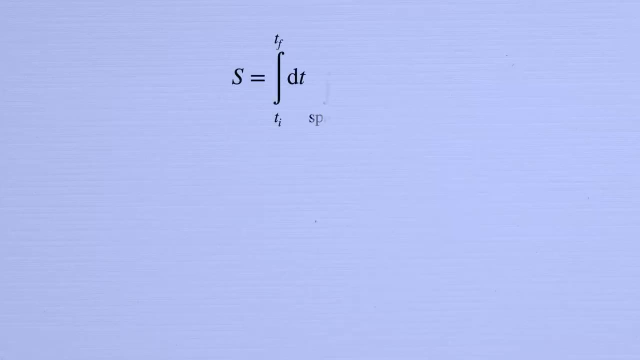 Next, we want to understand how all of this extends to a more general field theory, defined by its action given by integrating the Lagrangian density curly L over space and time. And, most of all, we want to understand how these conservation laws are related to symmetries by Noether's 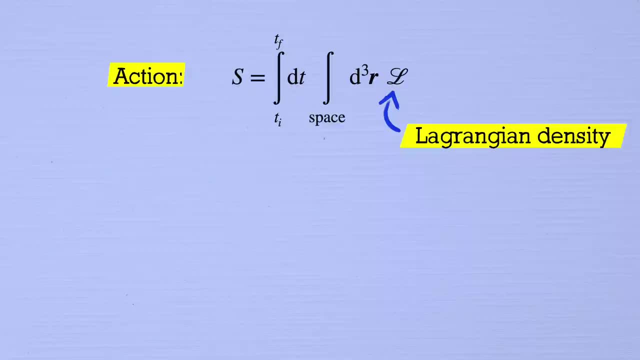 theorem. In particular, I hope you're really curious at this point to discover what symmetry is responsible for the conservation of electric charge. In the last mini-lesson video we studied the simplest example of a field theory called the Klein-Gordon theory. It consists of a single free field phi that assigns a number. 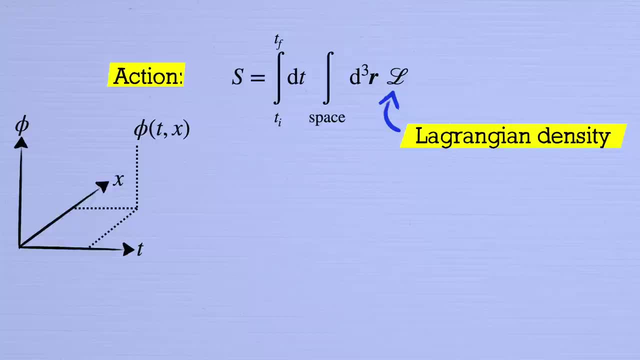 to each point in space at each time, And it's a great example for learning the fundamentals of field theory. It's defined by this Lagrangian density: 1 over 2 c squared d, phi by dt, squared minus half d phi by dx. squared minus half kappa squared phi, squared Plus the y and z derivative. 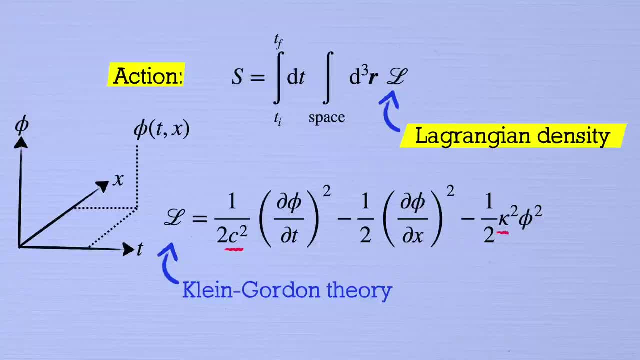 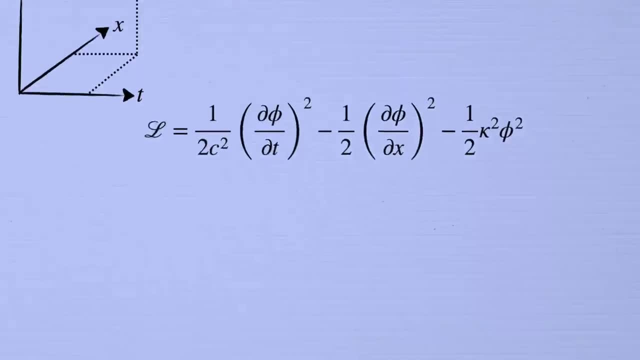 terms which I haven't written out. c here is the speed of light, and kappa is a parameter that we saw is related to the mass of the particles that you get when you turn this into a quantum theory. By applying the principle of least action to this theory, we found that the 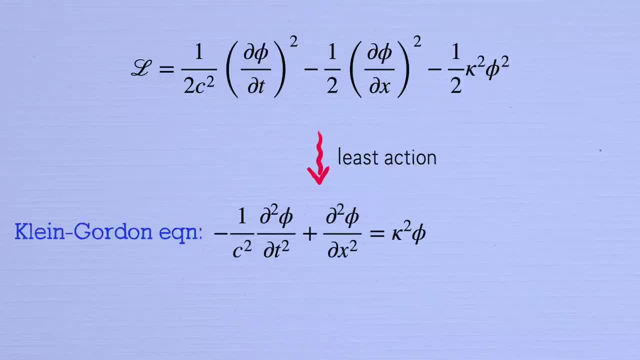 equation of motion for phi is this Klein-Gordon equation. It says that the second derivatives of the field with respect to time and space equals kappa squared times phi, which is a generalization of the wave equation. And we talked about how we can write the general solution of this equation. 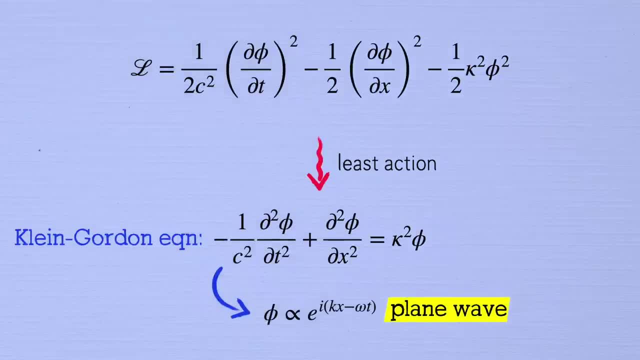 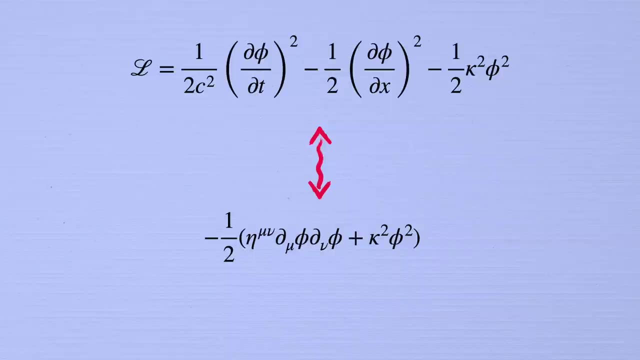 as a sum of plane waves. I also showed you last time how to write all this much more compactly with a relativistic notation. It makes all the formulas involved in this subject much more neat and concise, But on the other hand, if it's new to you then I think it might backfire and make 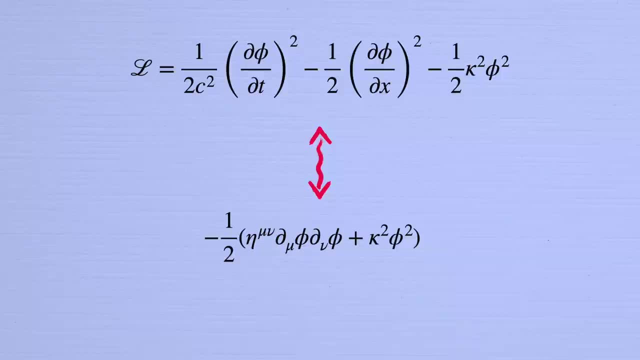 the equation seem mysterious. So first I'll work things through with all the t's and x's spelled out, And then afterwards we'll see how much simpler things look with a better notation. The catch is that we're going to have some very long formulas to deal with using the 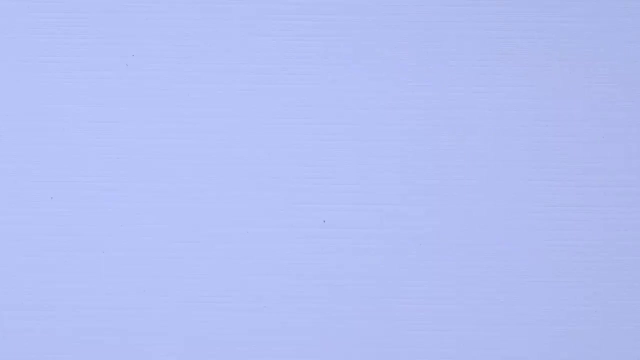 non-relativistic notation. Don't let them scare you off. When we talked about Noether's theorem for regular old particle mechanics, what we discovered was that whenever we had a symmetry of Lagrangian, meaning an infinitesimal transformation, that left it invariant. 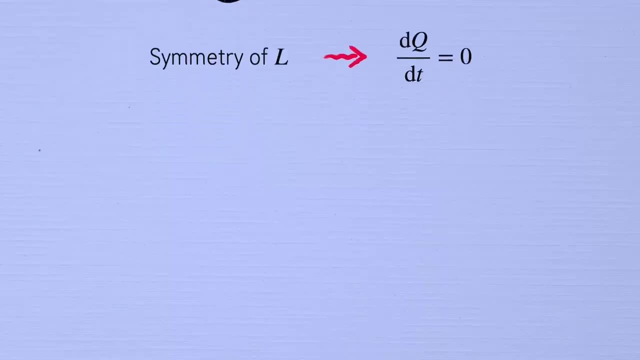 there would be a corresponding conserved quantity. For example, we looked at a problem with a block sitting on top of a flat, frictionless table attached to a spring that's pinned down at the other end. This setup does not have translation symmetry If you pick up the block and slide it. 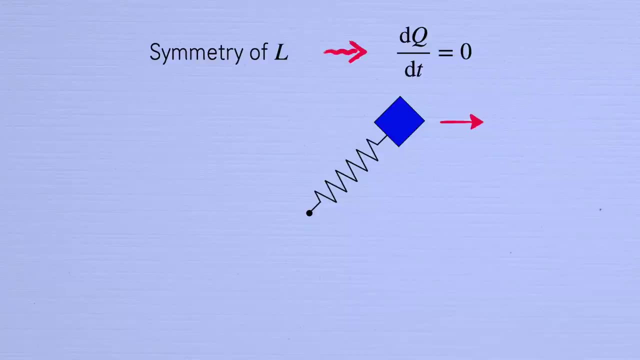 over to the right, say, the spring gets stretched and so you've changed the system. On the other hand, the system does have rotational symmetry, because you can pick up the block and rotate it around without changing the length of the spring. The potential for this is that the 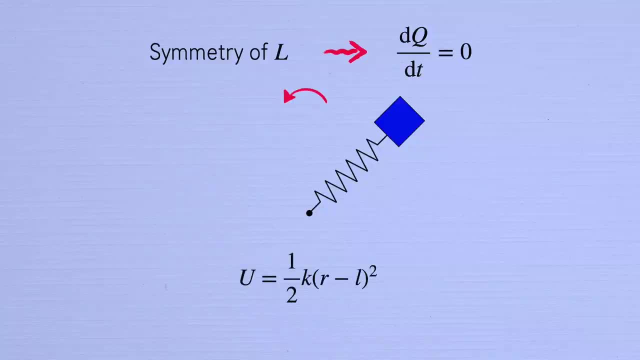 potential energy stored in the spring 1 half k times r minus l squared. only cares about how far away from the origin the block is measured by. r equals the square root of x squared plus y squared. It doesn't care about the angle theta that it makes. in the xy plane We showed that. 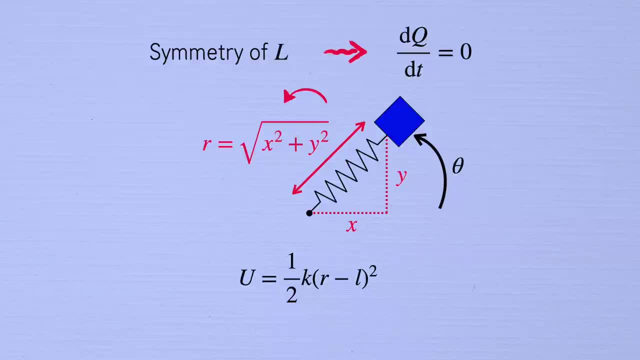 this rotational symmetry implies by Noether's theorem that the angular momentum of the block is conserved. We're going to discover a similar and even stronger relationship in field theory between symmetries and conservation laws. In fact, the simplest symmetry at the 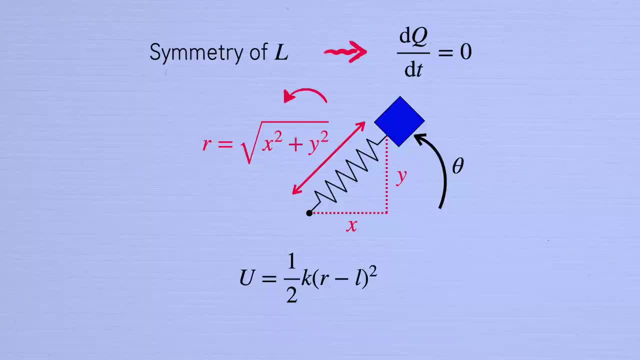 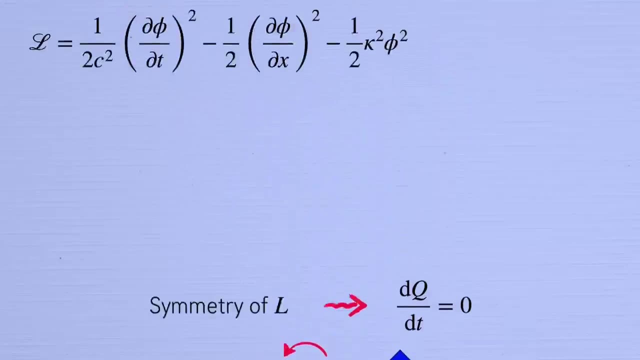 beginning of the standard model that's tied to electric charge conservation is closely analogous to the symmetry of the block on a spring. It's a rotational symmetry. but now in field space, To see how this works, it'll actually be more interesting. 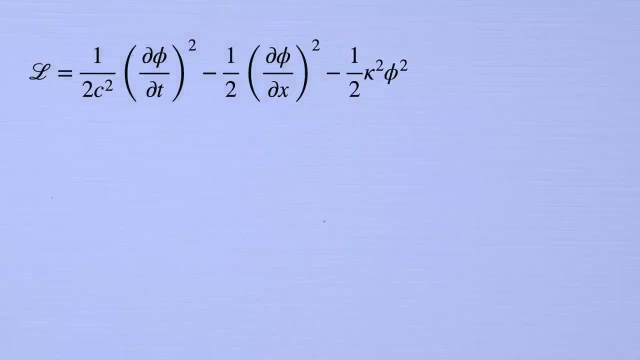 and more closely analogous to the field theory that describes the electron and electromagnetic force. to study a slight generalization of the Klein-Gordon theory, Instead of the real field phi that assigns a real number to each point in space at each time, let's consider a complex field that 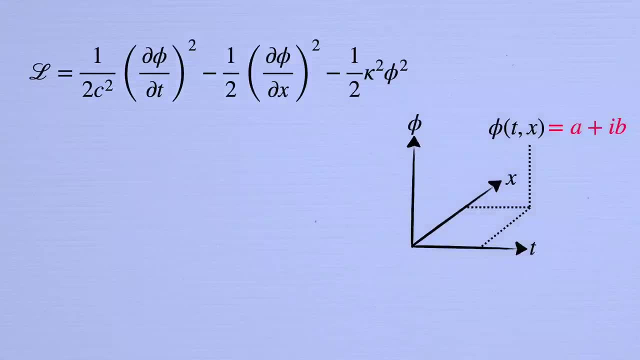 assigns a complex number to each point. Let's consider a complex field that assigns a complex number to each point. Let's consider a complex field that assigns a complex number to each point, meaning a number phi equals a plus i, b, with a real part and an imaginary part. 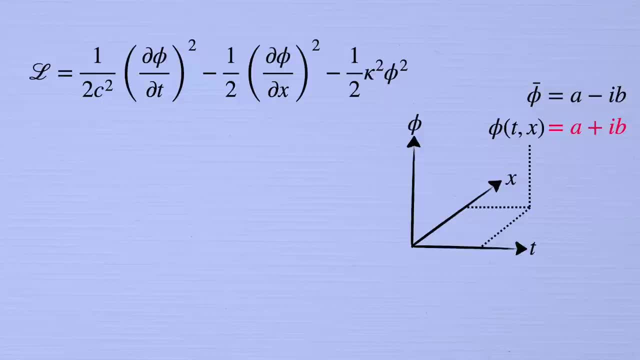 Write phi bar for the complex conjugate of phi, meaning a minus i b. Then we define the Lagrangian for the complex field like this: 1 over c squared d t of phi bar, d t of phi minus d x phi bar, d x phi minus kappa. squared phi bar phi, Where it's conventional to leave. 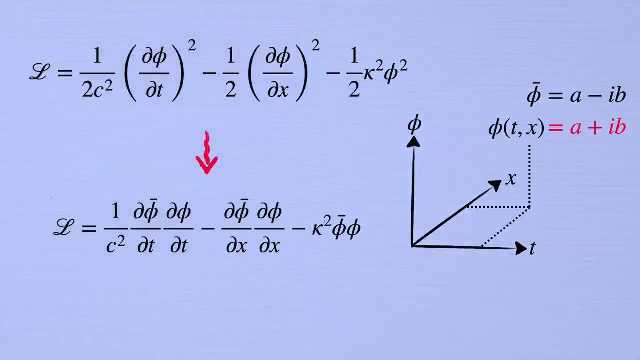 out the factors of half for the complex version. Despite the complex numbers, the Lagrangian is real because when you multiply a number by its conjugate, like in the last term here, you get a real number: a squared plus b squared. 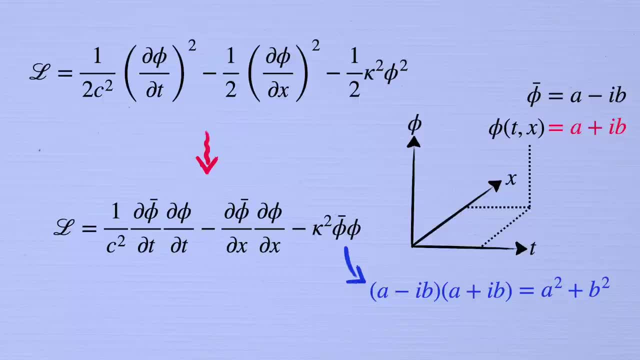 because the imaginary cross terms cancel out, and likewise for the other terms in the Lagrangian. If you split up phi into a real and imaginary part like this, then you can see that this new theory is actually just two copies of our old real Klein-Gordon theory, one for the real part. 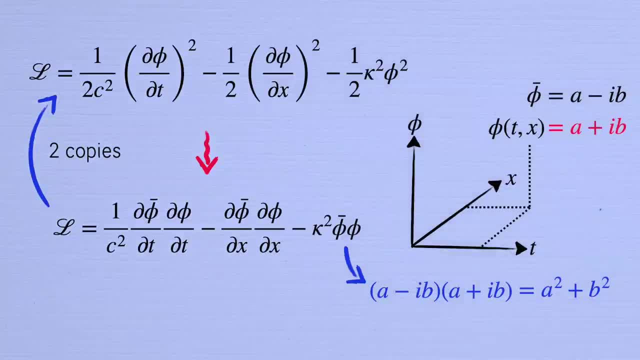 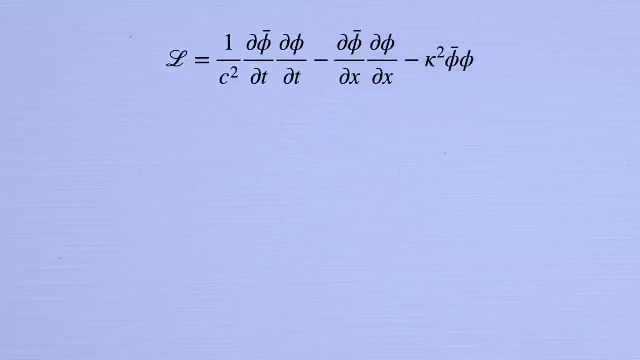 and one for the imaginary part. In the quantum version, we'll therefore get two kinds of particles, corresponding to a particle and its antiparticle. Now, what symmetries does this theory have? Like I mentioned, the one I want to focus on today is closely analogous to our block on a. 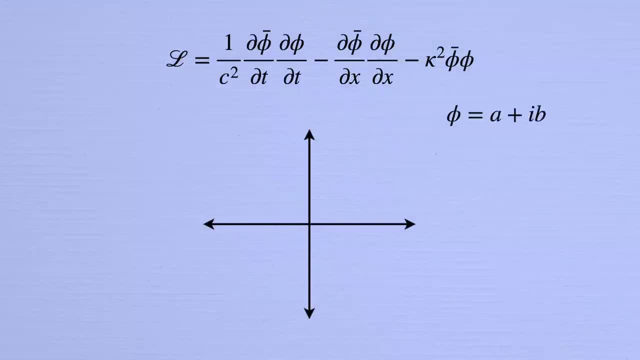 spring example from a minute ago. The real and imaginary parts of phi equals a plus i b. give us a point in a 2d plane with coordinates a and b. In other words, we can think of the complex number phi like an arrow that goes over to the right by a in the real direction and up in the imaginary. 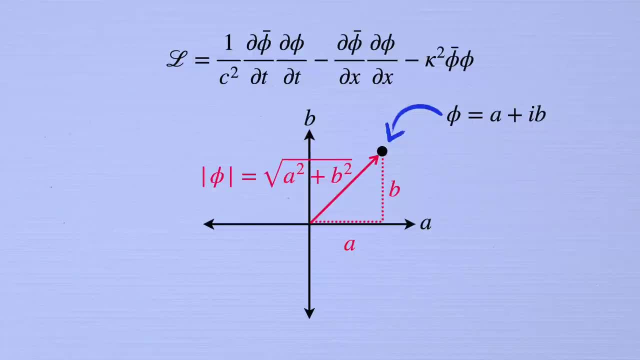 direction by b. The length of the arrow is the square root of a squared plus b squared, which I'll write as the absolute value of phi, also called mod phi, And it makes an angle theta with the horizontal axis. So just like in polar coordinates. 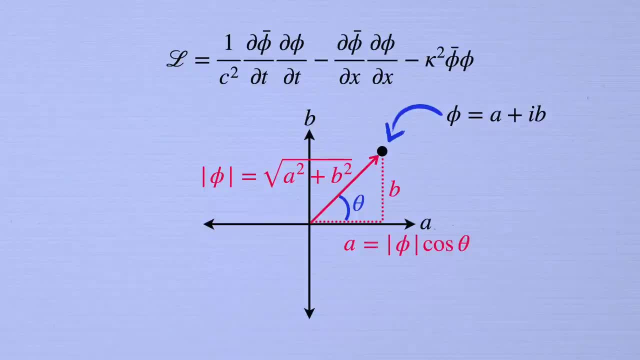 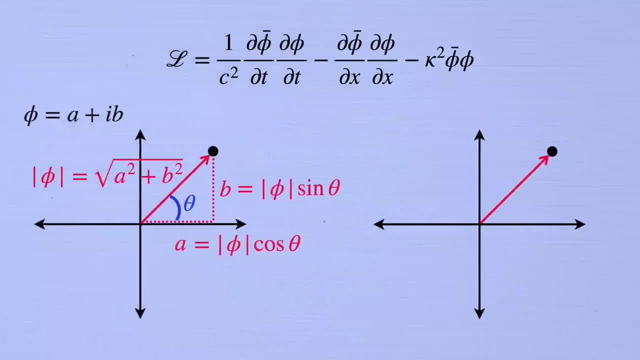 we can write the lengths of the two sides of the triangle as a equals mod phi cosine theta and b equals mod phi sine theta. But just like the block on a spring, our Klein-Gordon Lagrangian only depends on the length of the arrow, not on the angle theta that it makes in this plane. 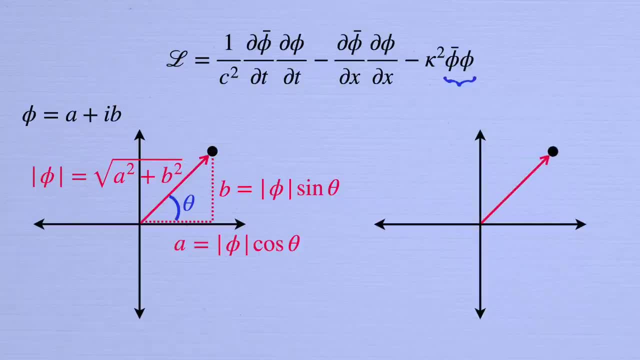 The reason why is that phi and phi bar always showed up paired together in each term of the Lagrangian. The last term, for example, is just phi bar. phi equals a squared plus b. The same goes for the terms with the derivatives, because, again, phi and phi bar always appear. 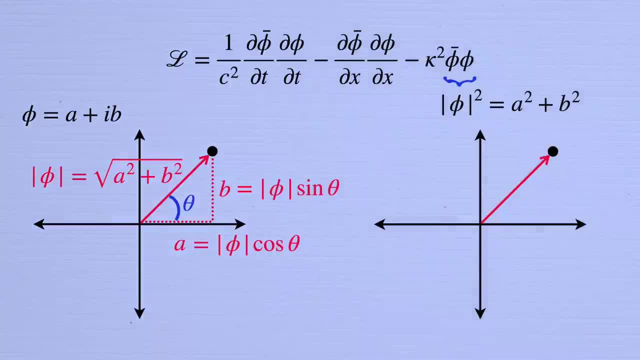 together. We therefore learn that this Lagrangian has rotational symmetry in the sense of the complex phi plane. This is the same kind of symmetry that leads to electric charge conservation in electromagnetism. Another way to say the same thing is to use the fact that a complex number 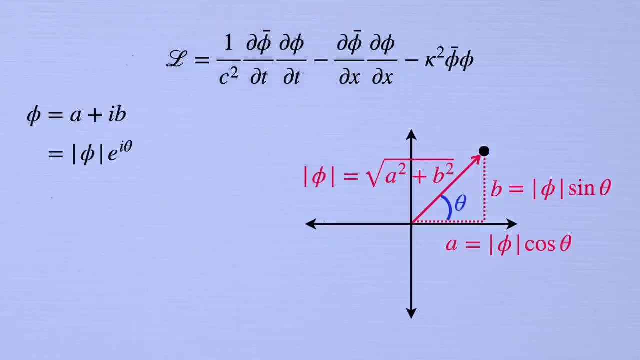 phi equals a plus i b can equivalently be written as mod phi e to the i theta. That's thanks to the fact that the integral of a plus i theta is a cosine theta plus i sine theta. So mod phi cosine theta and mod phi sine theta are just the horizontal and vertical components a and 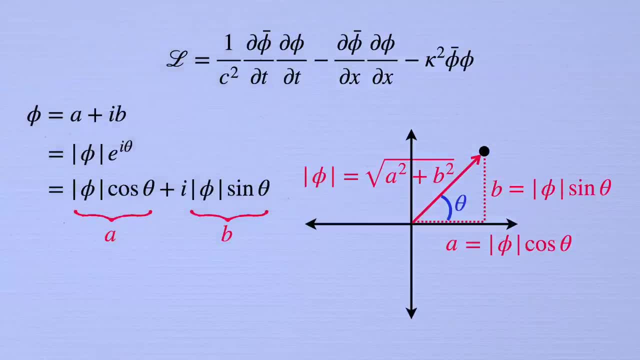 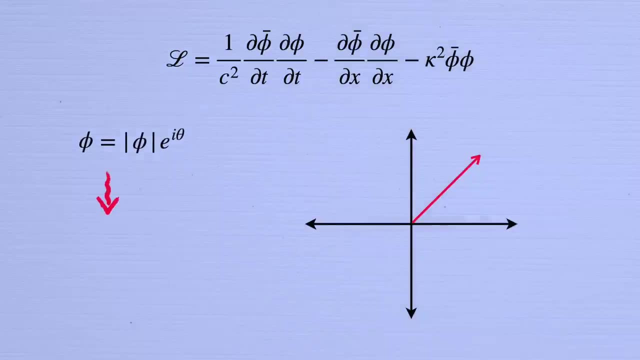 b of our arrow, And so this is the same thing as writing a plus i b. The reason why writing things this new way is convenient is that it makes it very simple to rotate phi to a new angle. Just multiply it by e to the i alpha for whatever angle alpha you want to rotate by. 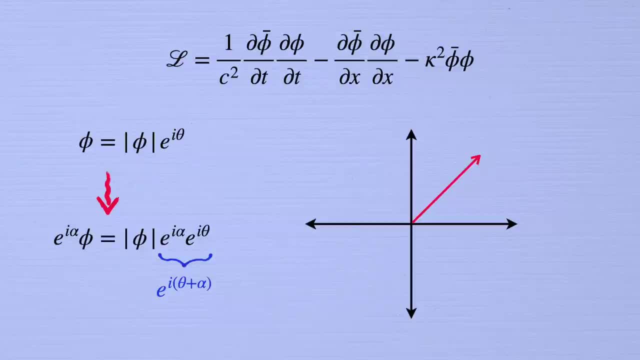 The things in the exponents, just add. And so, after we multiply it by e to the i, alpha phi gets rotated around to a new angle: theta plus alpha, But its magnitude doesn't change. The rotational symmetry of our Lagrangian is therefore simply the transformation. 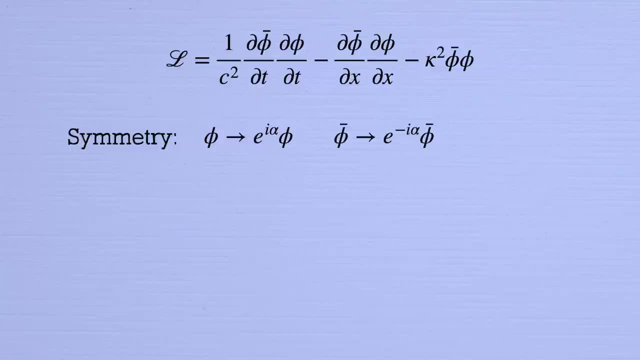 phi goes to e to the i alpha phi, and phi bar goes to e to the minus i alpha phi bar. And in this notation it's even easier to see why the Lagrangian is invariant, Since each term has a phi and a phi bar when we make the transformation. 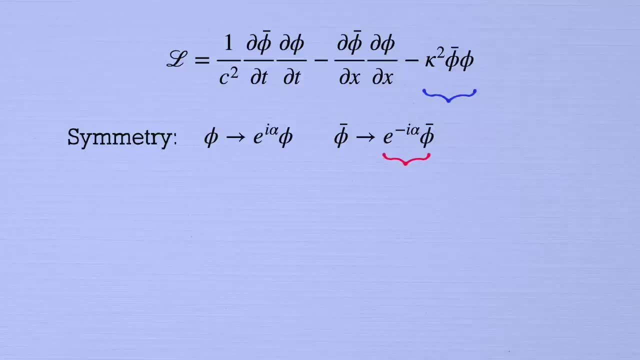 one picks up a factor of e to the i alpha and the other e to the minus i alpha, And when they're multiplied together they cancel out. This kind of symmetry is called u1, where the? u stands for unitary. The terminology comes from the definition of a unitary matrix. 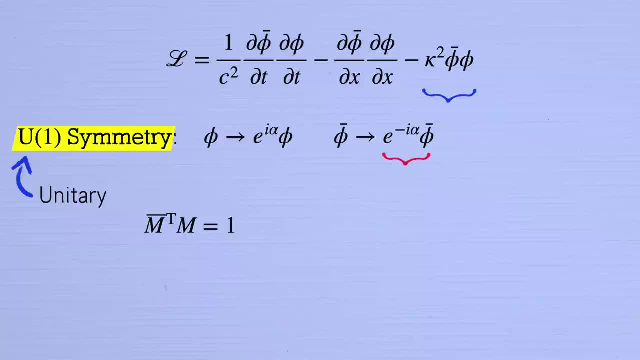 which is a matrix M that satisfies the property that if you take its complex conjugate and then its transpose you should get back the inverse of the matrix you started with The space of n by n matrices satisfying this property is called u of n, For n equals 1,. 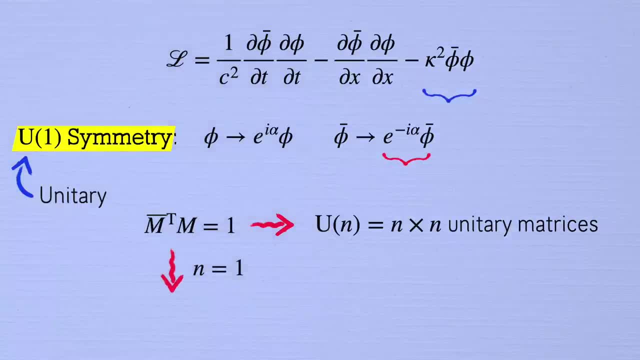 though the matrix is just a single number, and so the transpose doesn't do anything at all. In this condition, it's just z, bar z, or a complex number z, which is satisfied precisely by our rotation e to the i alpha. 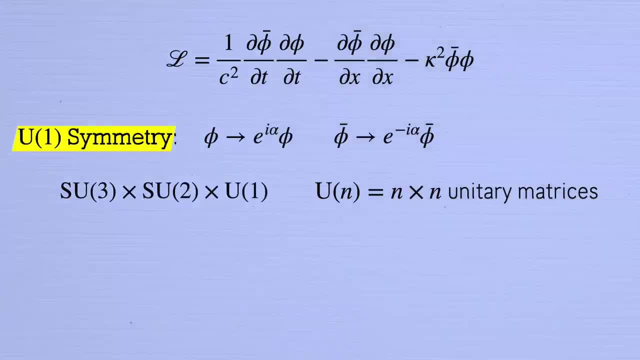 The other symbols in the standard model symmetry group- su3 and su2, stand for similar, larger symmetries, with n equals 2 and n equals 3.. The s just means that, in addition to being unitary, these rotation matrices are required to have determinant equal to 1.. 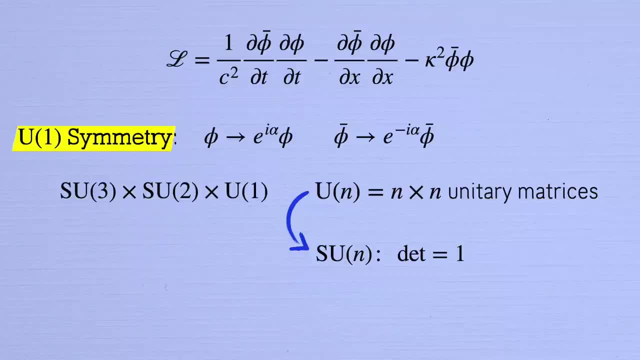 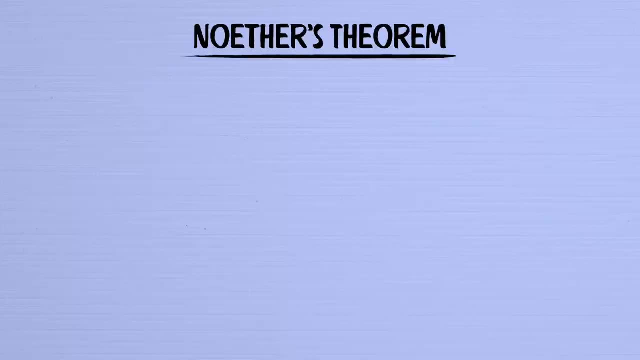 But we'll focus on understanding this u1 symmetry for this video. Now that we've identified it, we want to see how it leads to a conservation law by Noether's theorem. This is the basic way that Noether's theorem worked when we studied it before in particle. 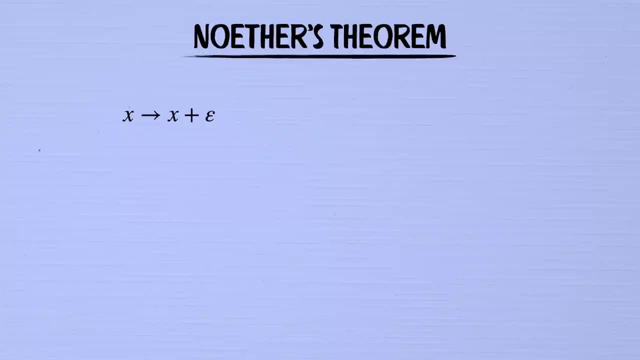 mechanics. The point was that under an arbitrary transformation of the coordinates, x goes to x plus epsilon, the change in the Lagrangian always takes the form: dl equals the equation of motion times epsilon plus d by dt of something. call it q. 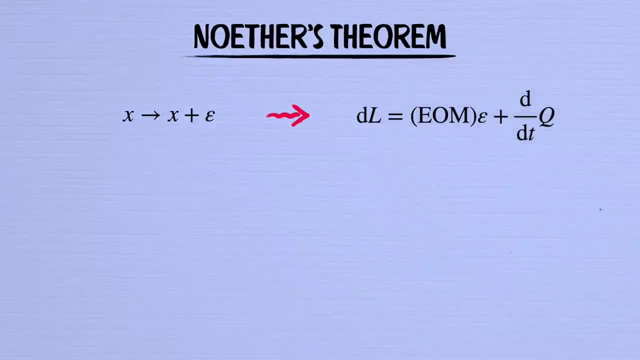 eom is the thing that vanishes when the particle is following its physical trajectory. If we choose a specific epsilon that gives us a symmetry of the Lagrangian, then dl is equal to zero on the left hand side, Then on the physical trajectory, where eom equals zero. this equation tells us that, whatever. 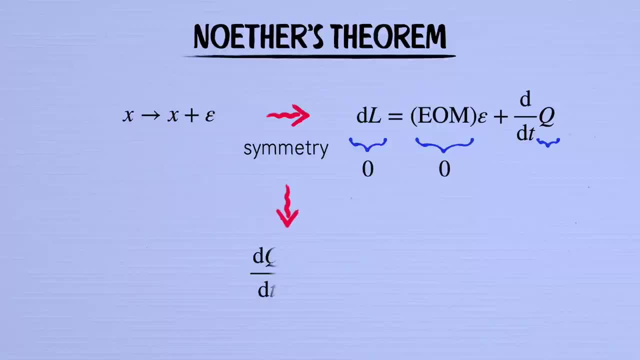 quantity q comes out for the particular transformation we picked will be conserved. dq by dt equals zero. So when we had a translation symmetry, q came out to be the momentum. When we had a rotation symmetry, it was the angular momentum, and so on We'll discover a very 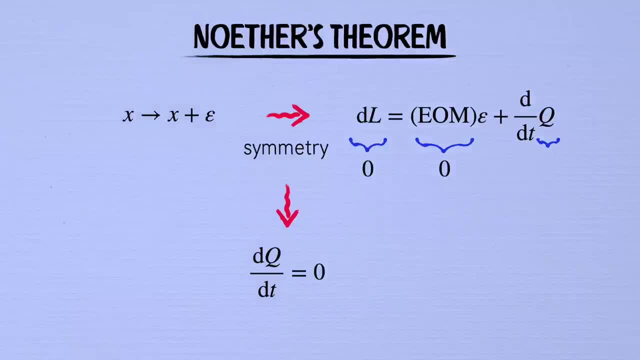 similar relationship in field theory. The main difference is that, because our fields now depend on both time and space, when we compute the change in the Lagrangian density we'll get both time and space derivatives on the right hand side For some quantities- rho and jx, jy and jz. 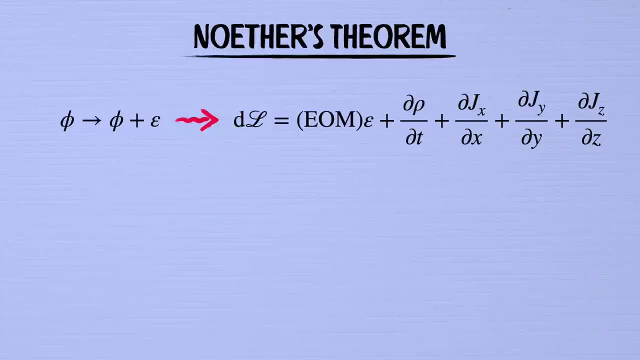 that'll depend on the transformation we're making. The argument is again that if we choose a specific symmetry transformation for which dl is equal to zero, then when the field is a solution of the equation of motion, we discover a continuity equation: d rho by dt plus del dot j equals zero. 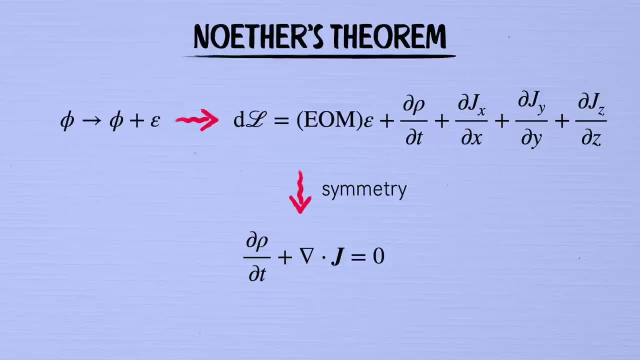 a local conservation law. This is the way Noether's theorem guarantees that symmetries lead to conservation laws in field theories. Now we're going to work it out for the rotation symmetry of our Klein-Gordon theory. We'll be running into some long equations for all the 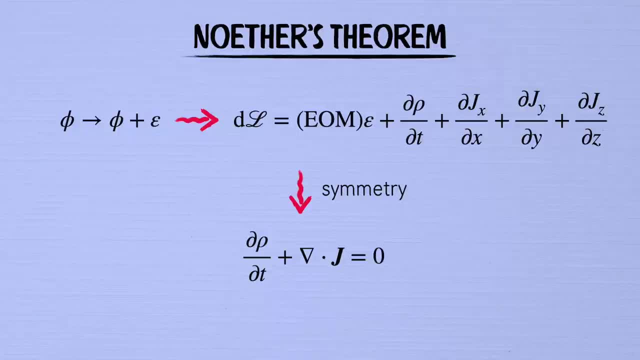 different ingredients here. If all this is new to you, then the most important thing on a first pass is to understand the shape of the argument, not to sweat all the details. When you are ready to iron them out, you can pull up the notes from the link in the description to take it step by step. 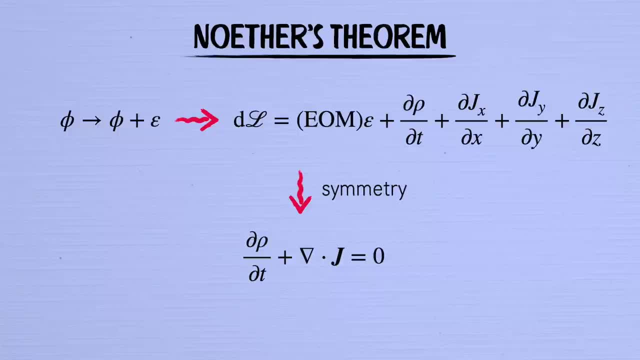 But for now just try to keep track of the basic idea. The change in the Lagrangian density always amounts to the equation of motion plus some time and space derivatives, And for a symmetry that gives us a local conservation law For the Klein-Gordon Lagrangian. we want to see how it changes when we make an arbitrary. 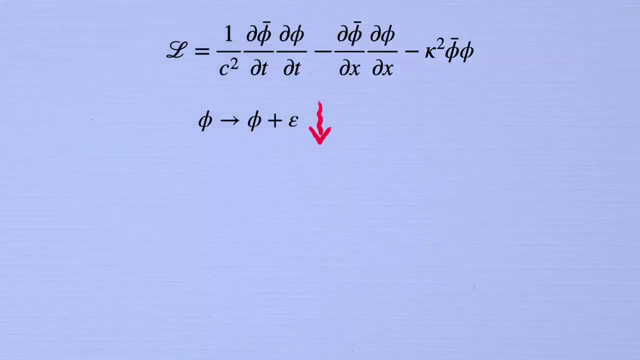 transformation of the field. phi goes to phi plus epsilon, where epsilon is an infinitesimal shift. It can be anything here, including a function of time and space and even phi itself For any random choice of epsilon. the Lagrangian certainly isn't going to be invariant If we make the 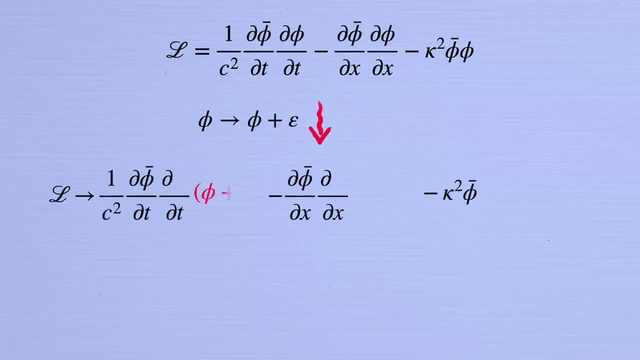 substitution, leaving phi bar alone for the moment. we get this new Lagrangian, These three terms with the phi's just give us back the Lagrangian we started with. The new pieces are the epsilons. Then the change in the Lagrangian under this transformation is: dl equals 1 over c. 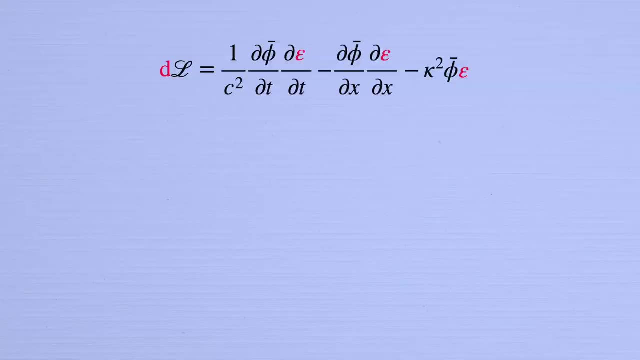 squared dt phi bar dt. epsilon minus dx. phi bar dx. epsilon minus kappa. squared phi bar epsilon. Next up. just like when we learned to apply the principle of least action, we want to integrate by parts on the first two terms, to grab the derivatives on epsilon and pull them over to. 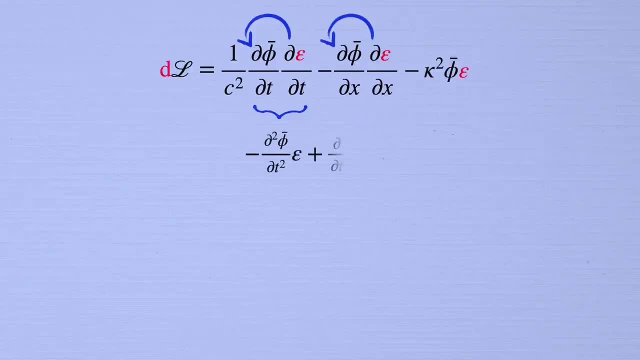 the other factor at the cost of a minus sign. So for the first term we get minus. the second derivative of phi bar with respect to time: Time is the derivative of phi bar with respect to time, Epsilon plus the time derivative of the whole thing. That's just an identity that we get by. 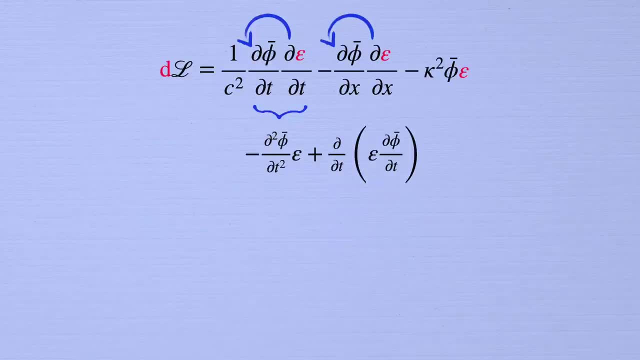 expanding out the derivative with the product rule, We can do the same with the x derivative term, and together we find that the leading change in the Lagrangian, when we make this tiny variation of phi, is given by this big expression. This looks like a lot. 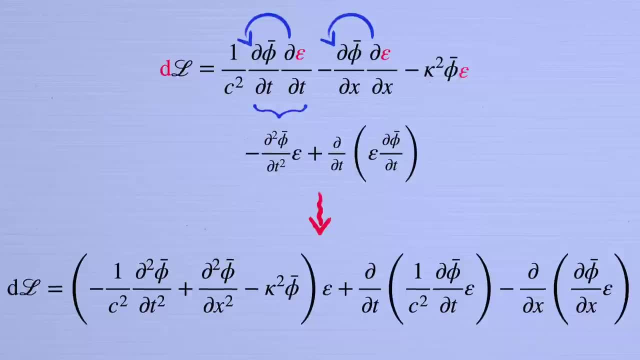 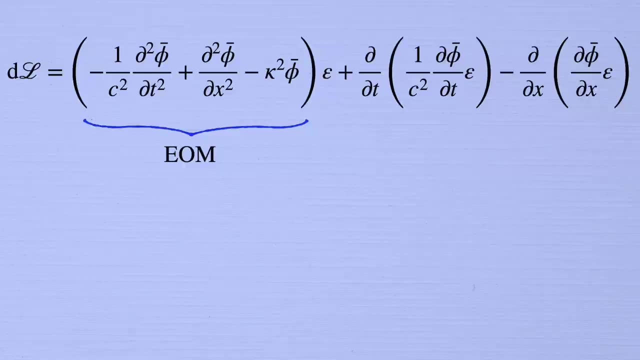 I can barely fit the thing on the screen, but remember, the idea is pretty simple. This is just what we predicted for dl from a moment ago. The first big quantity in parentheses is just the thing that vanishes when phi bar satisfies its Klein-Gordon equation. 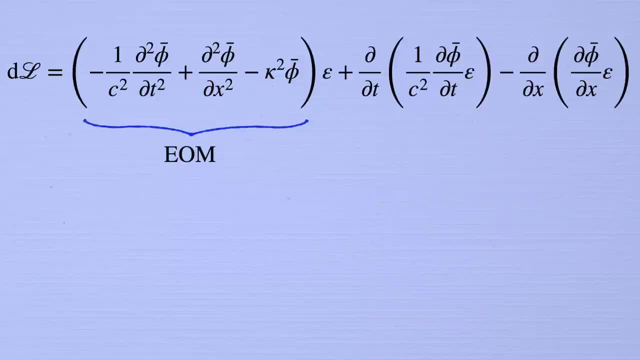 Then on top of that, we get some time and space, derivative terms Indeed, this was almost exactly the procedure we followed last time to derive the Klein-Gordon equation by applying the principle of least action. The only difference was that in that case, we required epsilon to 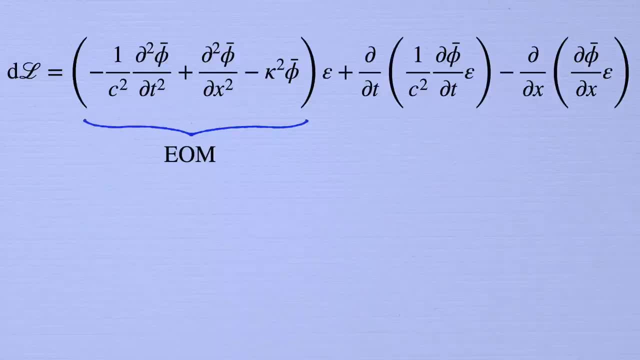 vanish at the boundaries of the action integral. But our identity here for dl holds for any transformation. phi goes to phi plus epsilon And of course phi bar will also transform as well. in general, phi, phi bar goes to phi bar plus epsilon bar. That works out in a totally analogous. 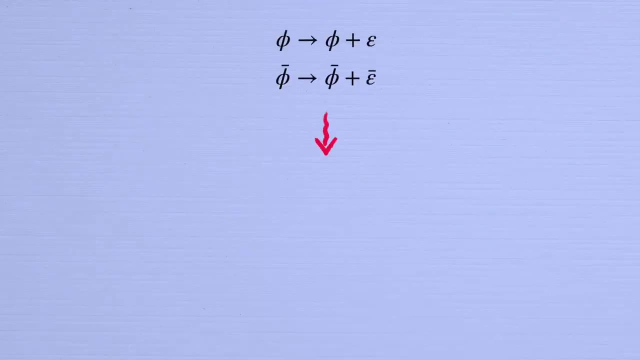 way, And that's what we're going to do. next. We're going to apply the principle of least action to dy And when we add it all up to find the total change in the Lagrangian, we get an equation of the form we expected. dl equals terms with the equations of motion plus d rho, by dt plus dx jx. 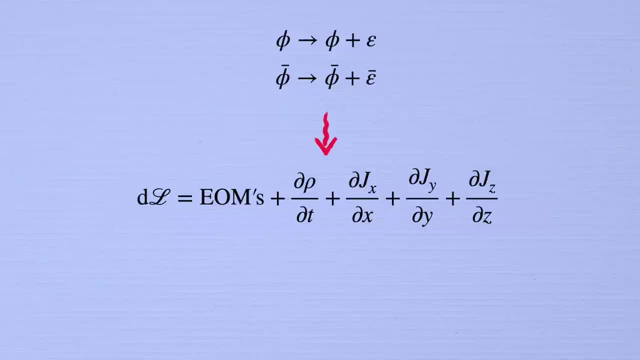 dy, jy and dz jz, Where I have to find rho to be 1 over c squared. epsilon dt phi bar plus epsilon bar dt phi and jx equals minus epsilon dx phi bar plus epsilon bar dx phi, And similarly for jy and jz. 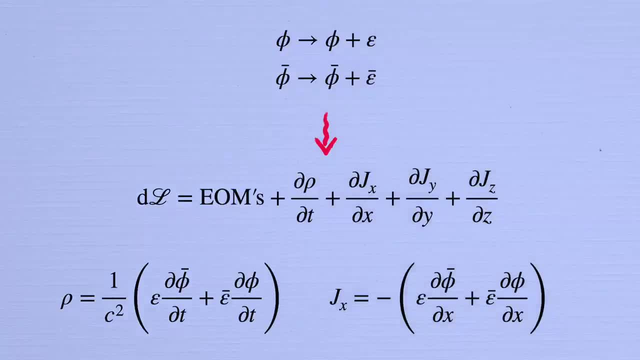 And don't worry, these aren't supposed to look as special, especially intuitive at this point. But Noether's theorem is now staring us in the face. This formula for dl holds for any transformation. But if we now choose a specific symmetry transformation for which dl equals zero, then when the Klein-Gordon equations are satisfied, 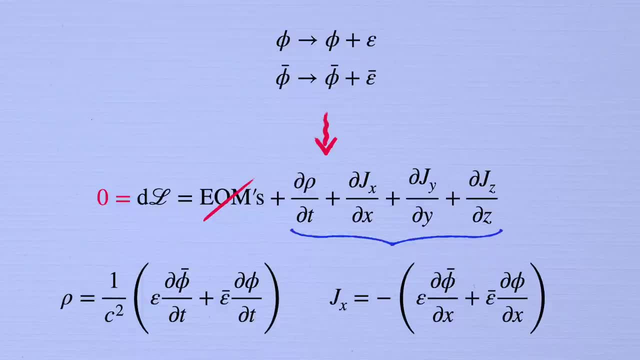 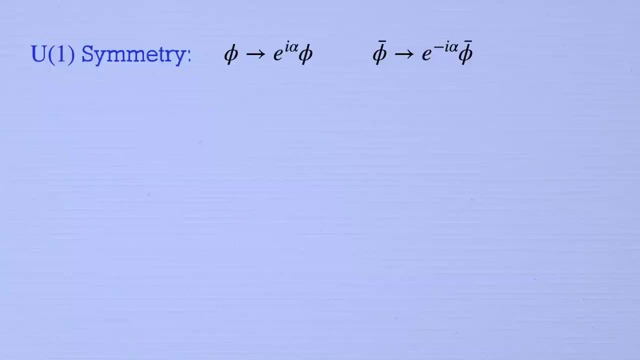 we learn that the corresponding rho and j define a conserved charge and current. So now let's plug in our rotation symmetry. It's a symmetry for any angle alpha. But to apply Noether's theorem, we only care about the infinitesimal version. So let's apply the 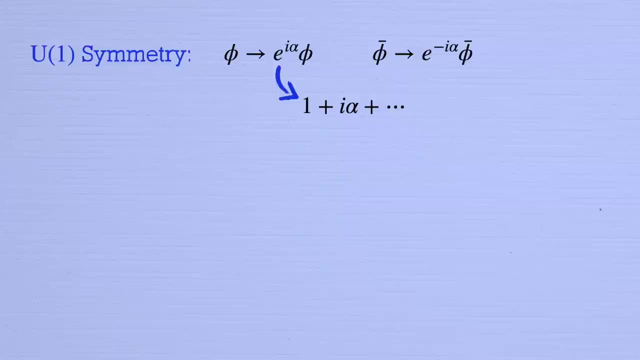 Taylor series e to the i alpha And then apply the Taylor series e to the i alpha Equals 1 plus i alpha, plus dot dot dot, Where we only need to keep the first interesting term. Then our infinitesimal rotation symmetry sends phi to phi plus i alpha phi. 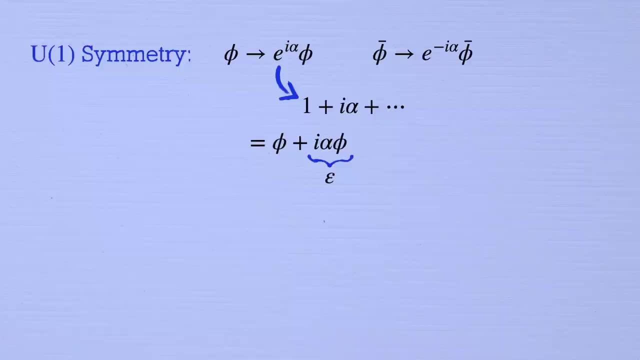 meaning that epsilon is equal to i, alpha, phi, And likewise for phi bar. When we plug this epsilon in to our formulas for rho and j, we find that the rotation symmetry leads to a local conservation law with this charge density and this current density. 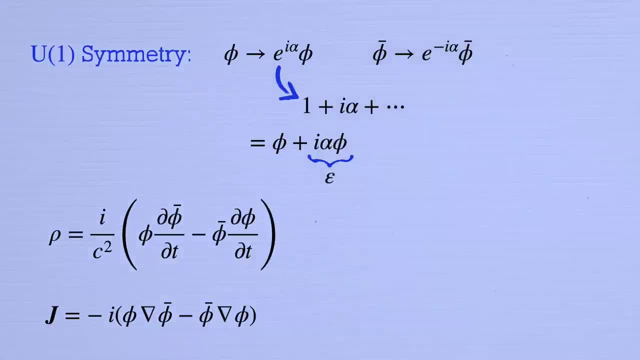 I've dropped the overall factor of alpha here because that was just an arbitrary constant. Don't sweat the i's. by the way, The things in parentheses are pure imaginary, since they're each a complex number minus its complex conjugate. Then multiplying by the i. 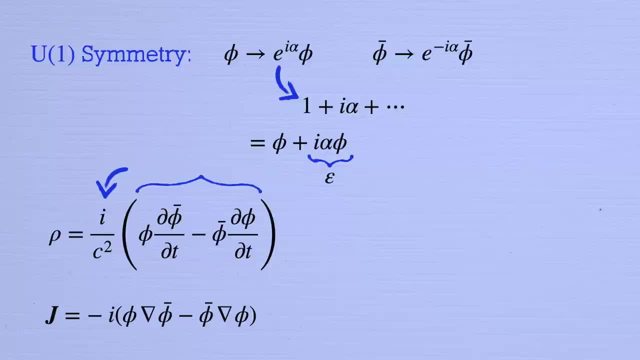 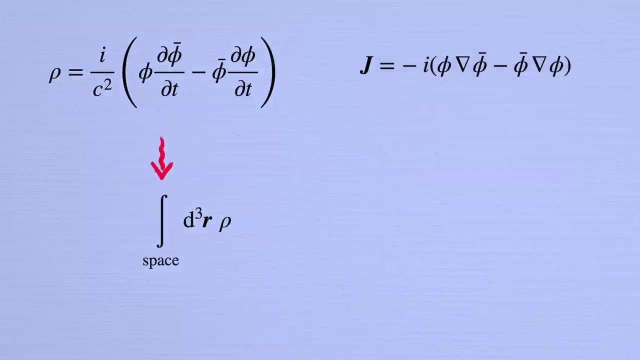 out front gives us back a real number, Since this transformation was a symmetry. Noether's theorem implies that rho and j satisfy the continuity equation, And we've discovered a conservation law. But a conservation law for what? What do these formulas mean? Well, remember that the conserved charge is defined by integrating the charge. 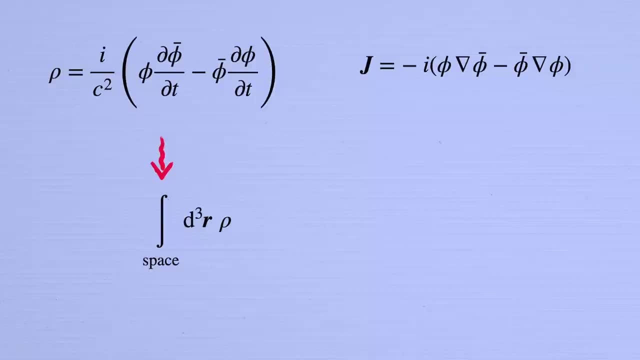 density rho over space. Also recall that last time we decided that the charge density was going to be equal to the total charge density rho over space, And that's exactly what we're going to do. The general solution to the Klein-Gordon equation can be written as a sum of plane waves. 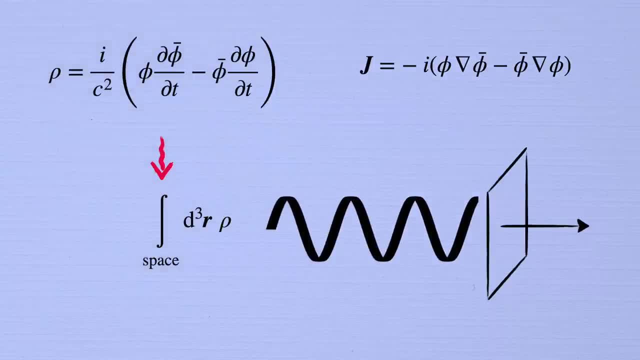 And these turn into wave functions for the particles created by the fields in the quantum theory. By plugging that expansion into this integral, you can show that what it does is count the number of particles minus the number of antiparticles. Suppose these particles carry. 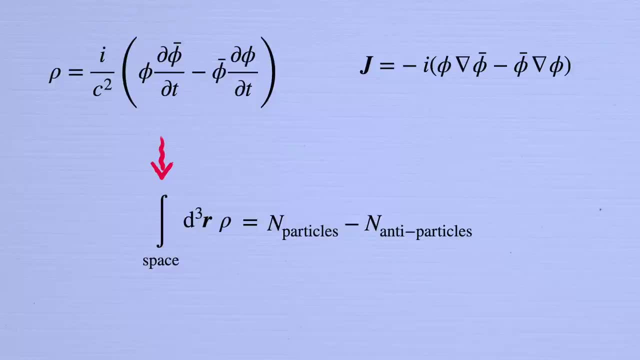 electric charge q and therefore the antiparticles carry electric charge minus q. Then the total electric charge is q times the number of particles minus the number of antiparticles. In other words, it's our conserved quantity here, given by integrating rho up to a factor of q. 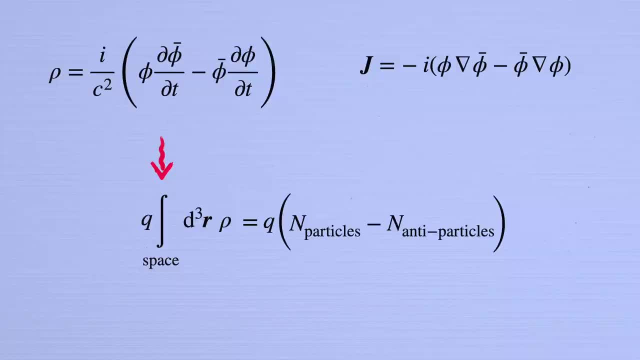 So the same conserved quantity coming from our rotation symmetry counts the total electric charge. The densities rho and j from the rotation symmetry essentially become electric charge and electric current densities. But once we start talking about things with electric charge that means that in addition to our field phi there are electric and magnetic fields floating. 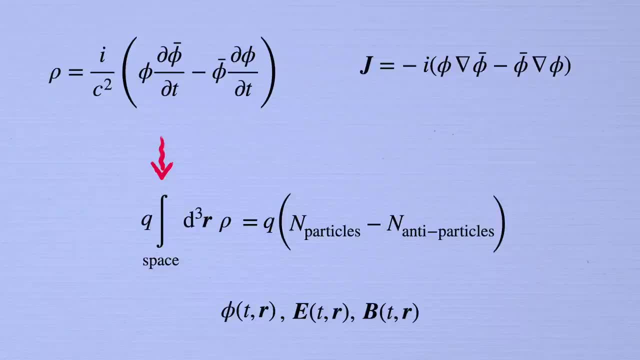 around as well, And our field theory had better incorporate all of them. In the last part of the video, I want to show you the Lagrangian-Helmholtz equation. I'm going to show you the Lagrangian-Helmholtz. 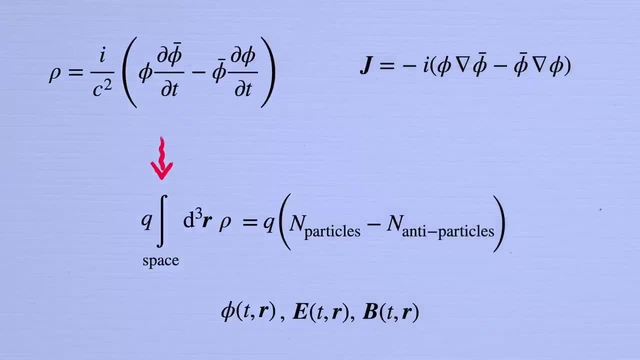 equation and then I'm going to show you the Lagrangian-Helmholtz equation. But before we do that I want to show you the Lagrangian for the full theory, including the electromagnetic fields. To do that, it's going to be really useful to switch to the relativistic notation we talked. 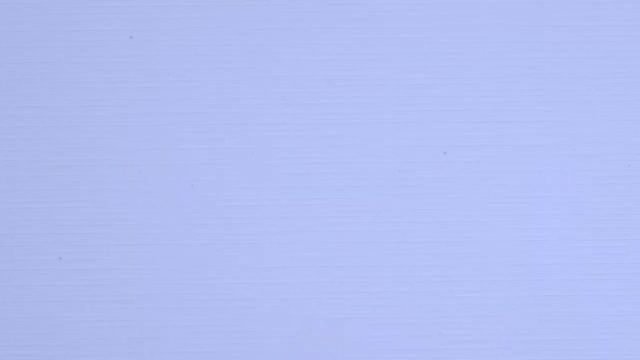 a little bit about. in the last field theory video I showed you how to write the spacetime coordinates as a four-component vector: x, mu. where mu equals zero, one, two or three is an index. Mu equals zero is the time component. x. zero equals c, t And mu equals one, two, three. 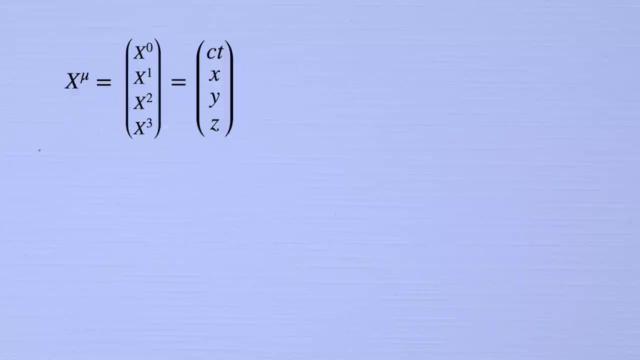 are the space components x, y and z. That factor of c is there so that all the entries have the same dimension, And that's what we're going to talk about in this video. So let's get started. Then we can define the derivatives with respect to x, mu by d by dx. mu equals one over c, d by dt. 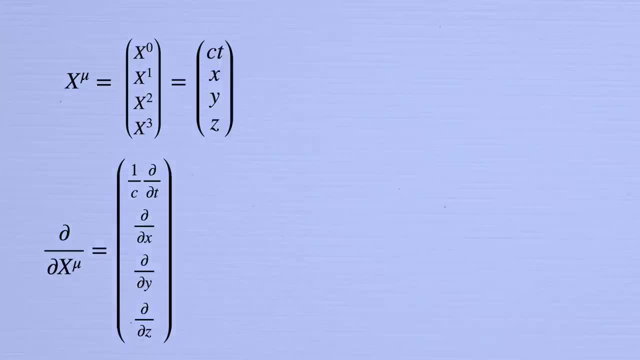 d by dx, d by dy, d by dz, And we usually write this even more simply as d sub mu. We can likewise put the charge density, rho and the spatial current j together into a four-component spacetime current j, mu. The c is again there, so that each component has the same units. 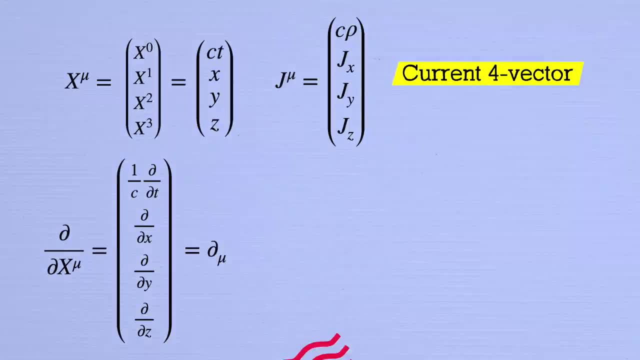 This actually makes a lot of sense. The spatial current density j vector is the amount of current flowing around through space, while c times rho is like a current flowing forward through time, Even if you just set a charged particle down at rest, so that the spatial current is zero. 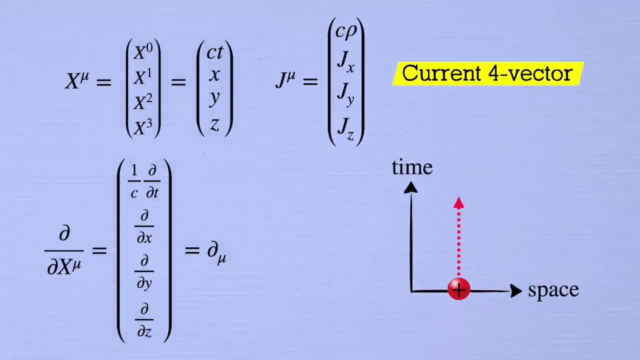 the particle is still moving forward through time as the clock ticks onward and c? rho is measuring the spacetime current in that direction. In this notation, the continuity equation simply says that the sum over mu, of d, mu, j, mu is equal to zero, Because if we expand it out, we get d zero, j zero, which is one over c, d by dt of c. 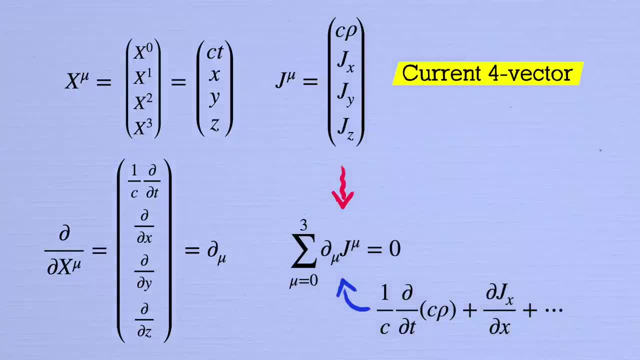 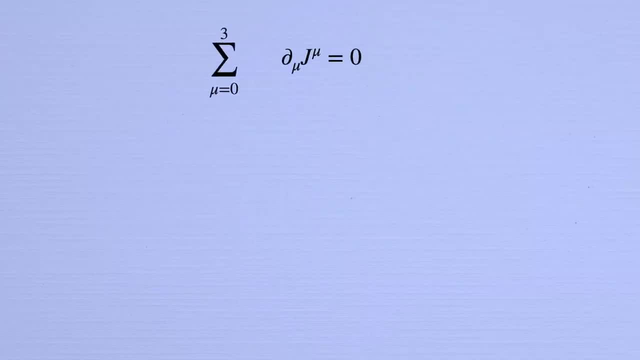 rho plus dx, j, x, dy, j, y and dz, j z, Just like we had before. In fact, we usually don't even bother to write out the sum symbol. We just adopt the convention that any time an index like mu appears twice in any given term, like it does here, 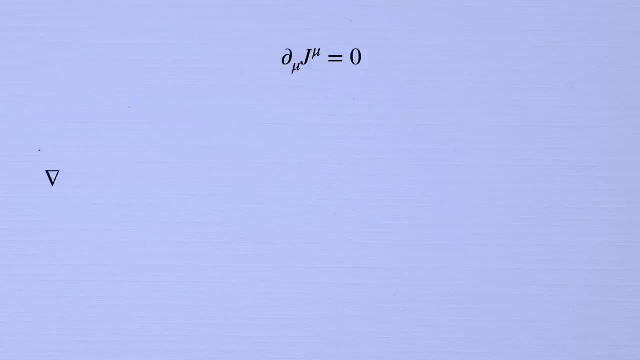 then we sum over all of its values. The spatial divergence del dot j measures how much j spreads outward from a given point in space, like a water sprinkler spraying water out of a spigot. The continuity equation says that j? mu can't have any. 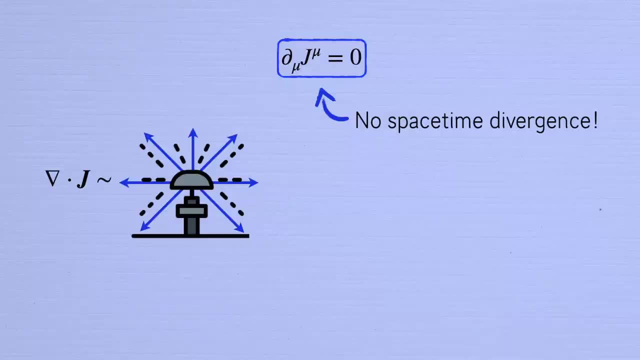 divergence in spacetime, meaning you're not allowed to simply pop out new electric charges at any spacetime point, or at least no net charge. Now I want to use this powerful notation to write the Lagrangian for the full theory, including the electromagnetic fields, Really getting into. 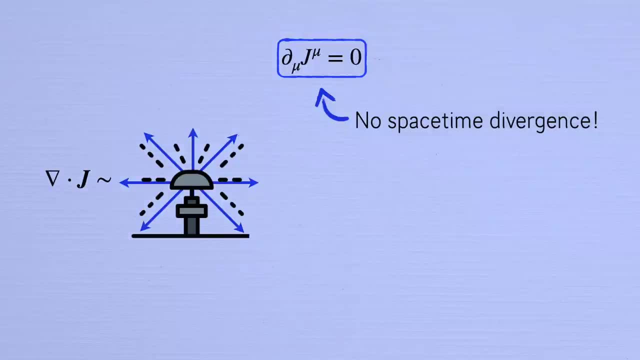 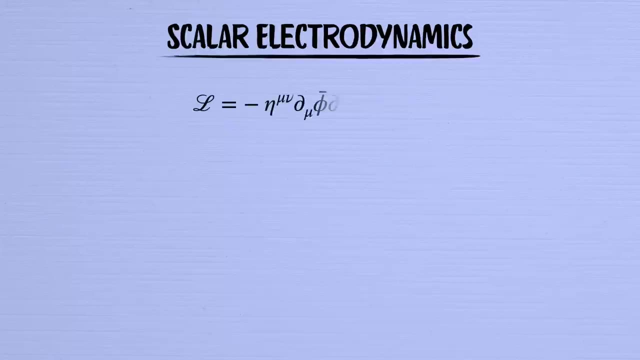 all the details here would deserve a video of its own, or several. So for now I'm just going to give you a quick sketch of the different ingredients and how they fit together In our relativistic notation. we can write the Klein-Gordon Lagrangian much more compactly. 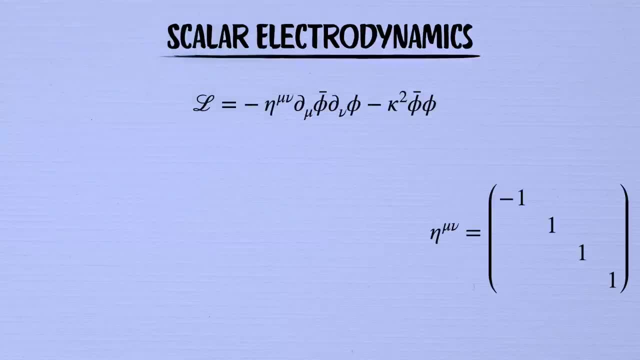 like this, Where eta is another bit of notation we defined last time. It's a 4x4 diagonal matrix with minus one in the top left corner and ones for the rest. It just serves to take care of the relative minus signs for us between the time and space terms Because, remember, it's implied that 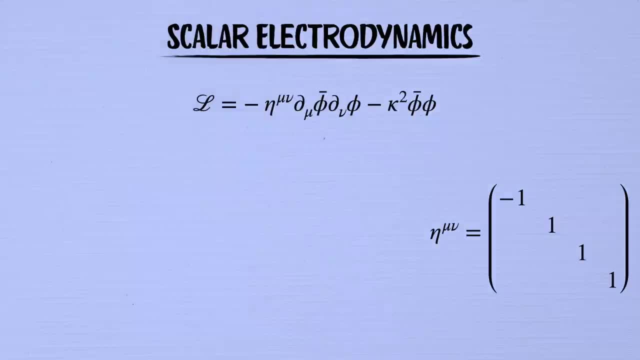 we're summing over both mu and nu here. When we expand out the sum, we get the same Lagrangian as before, and that'd be good practice for you to check for yourself. to get more comfortable with this abstract notation, I'm also going to work in units where c equals 1. for the rest of the video, since that's the only way to do it, I'm also going to work in units where c equals 1 for the rest of the video. since that's the only way to do it, I'm also going to work in units where c equals 1 for the rest. 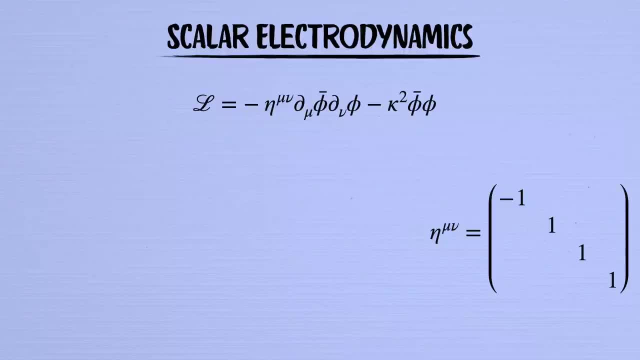 the standard colour convention field theory and it makes the formulas look a lot simpler. As we've seen, L is invariant under the U1 rotational symmetry, where I've inserted a factor of q in the exponent, since that's going to become the electric charge. 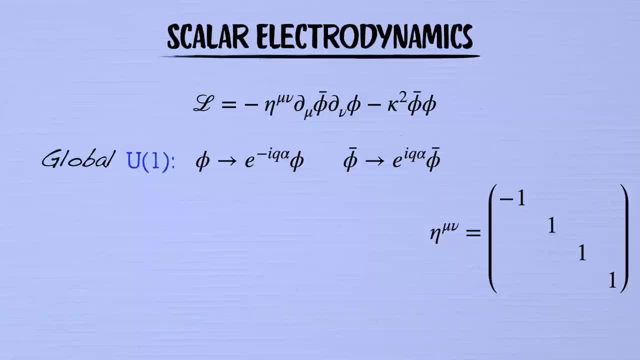 in a second. This is a global symmetry, meaning that the angle Alpha is a constant. We're performing the same rotation of the field at every point in space-time. But electromagnetism and the Standard Model as a whole are examples of gauge theories. 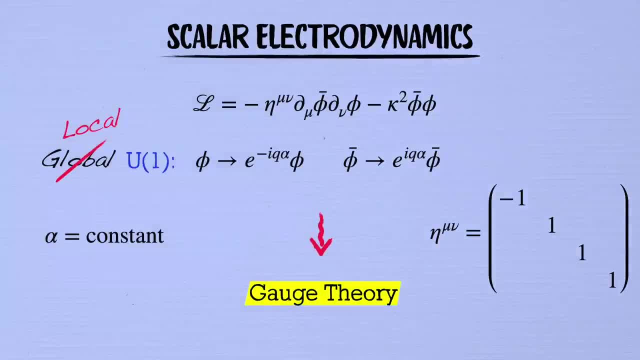 in which the defining symmetries are promoted to local transformations in spacetime. In other words, the U1 gauge symmetry of electromagnetism is obtained by demanding that the Lagrangian is invariant under this rotation for any choice of alpha of x. 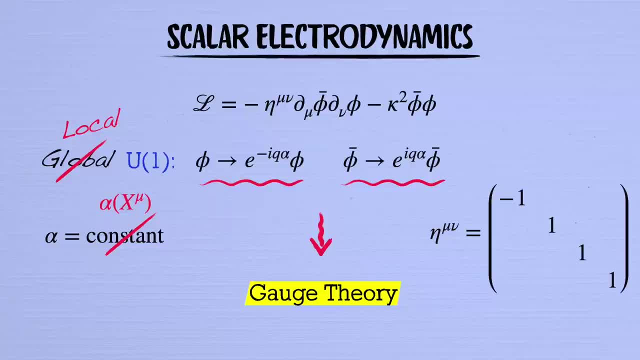 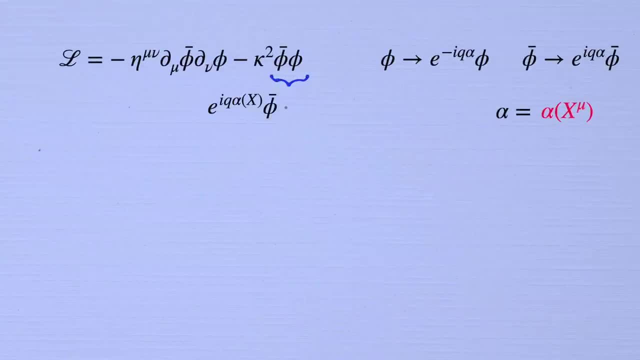 including one that depends on what point you're at in space and time. Our original Lagrangian is not invariant under rotations when alpha is a function of x. The second term is still okay because the two rotations coming from phi and phi bar cancel each other out. but the terms with the 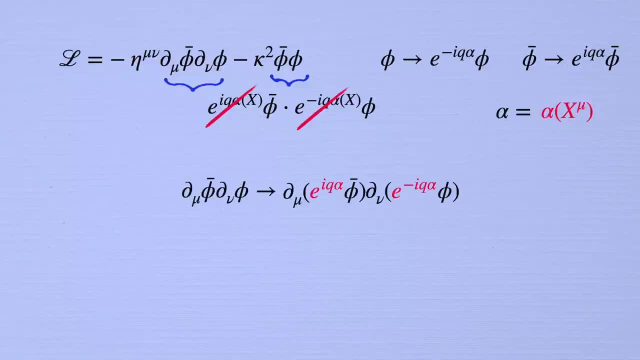 derivatives are no longer invariant. When alpha was a constant, we were able to pull those rotations right outside the derivatives and then they cancelled against each other and left the Lagrangian unchanged. But when alpha of x becomes a function of x, we'll get additional terms from. 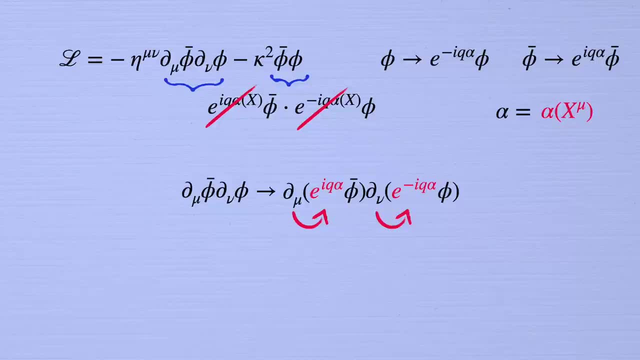 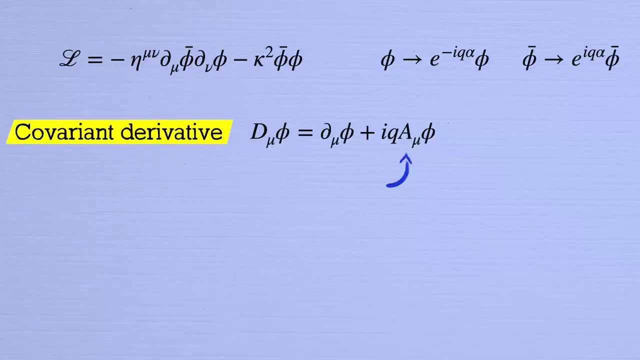 the product rule when the derivatives hit the alphas and these do not cancel out. The way to resolve this problem is to replace these ordinary derivatives with what's called a covariant derivative. It's defined by the regular derivative of phi plus iq, amu, phi, where amu is a new field, the electromagnetic potential. 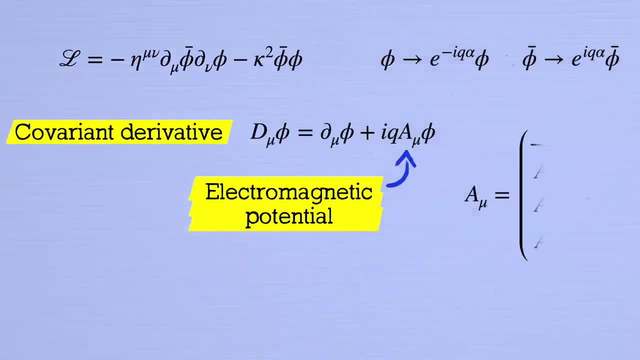 And you've almost certainly met at least part of it before. It's another four-vector with the regular old electric potential in its first slot, in other words the voltage, and in the spatial slots is the magnetic vector potential which is needed in addition to v. 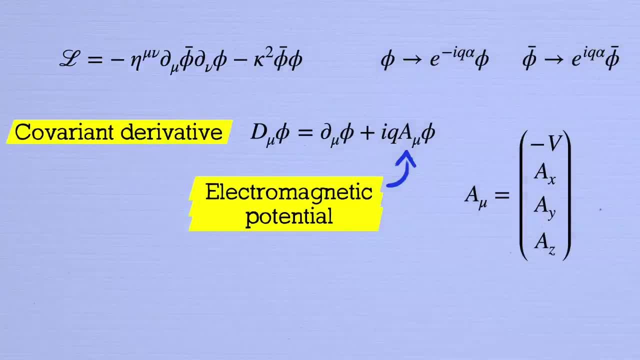 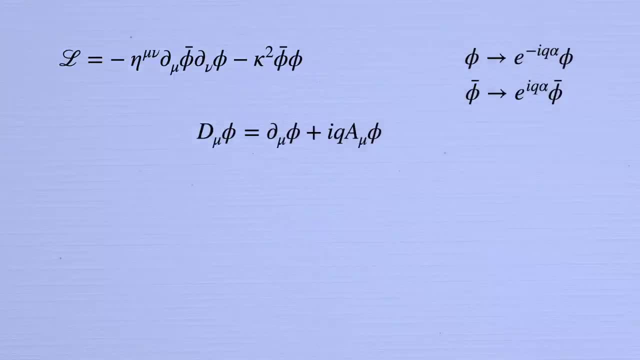 once magnetic fields are thrown into the mix, They're related to the electric and magnetic fields by taking a few derivatives. I'll hopefully go through those details in a later video. What this covariant derivative does for us is restore the nice transformation property that leaves the Lagrangian invariant. 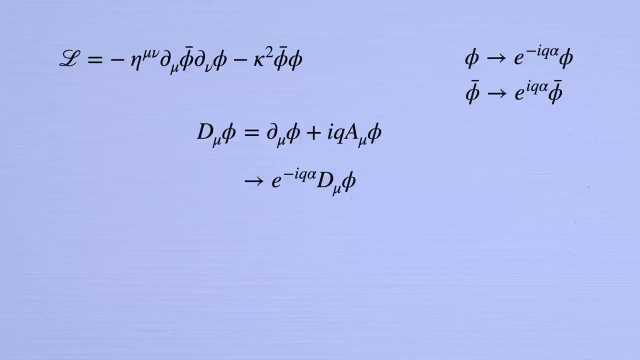 even when alpha is a function of spacetime, Provided that when our transformation rotates phi and phi bar, it simultaneously sends a to a plus d alpha. This is called a gauge transformation and it reflects the fact that the electromagnetic potential isn't uniquely defined. 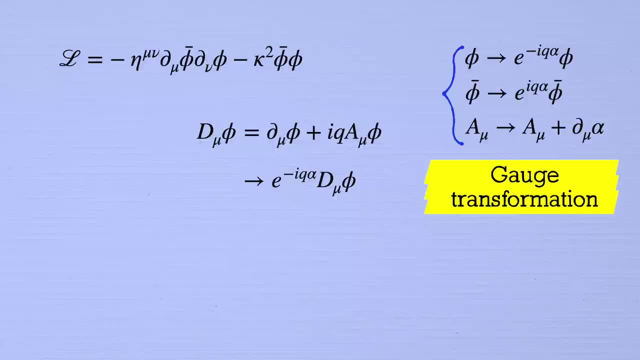 Different choices for a mu related by gauge transformations will describe the same electric and magnetic fields. I'll leave it as a little exercise for you to check this transformation property. The upshot is that if we replace the ordinary derivatives with covariant derivatives in our original Lagrangian we get a theory that's invariant even when alpha is a function. 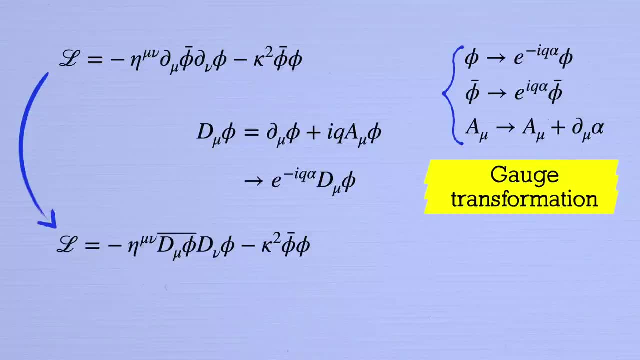 of spacetime, because the rotations again come outside the derivatives and cancel each other out. The result of this procedure, which just looks like a trick at first glance but has deep theoretical underpinnings, is that the field phi now carries electric charge. q. 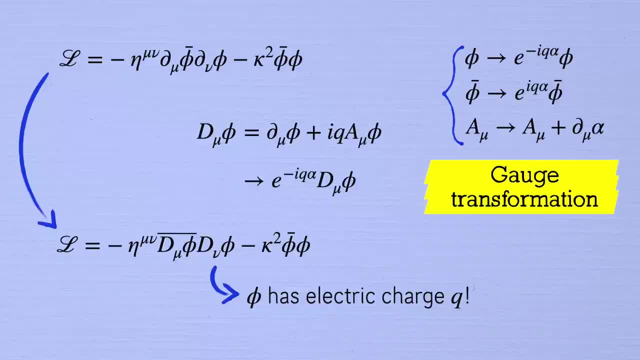 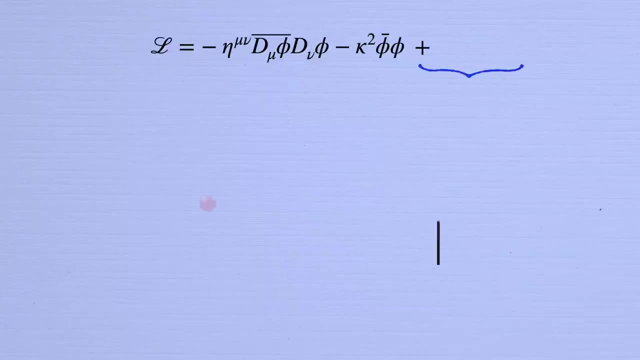 and phi bar carries charge minus q. The noether current is now a source for the electromagnetic field, Just like any electric charges and currents would produce electric and magnetic fields, according to Maxwell's equations. But speaking of Maxwell's equations, there's still one thing missing from our Lagrangian Maxwell's equations determine: 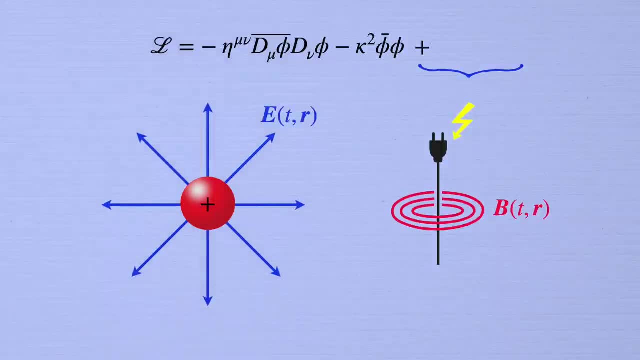 how electric and magnetic fields are produced by charges and currents and how they evolve with time. They're the equations of motion for the electromagnetic potential. a mu, Just like the Klein-Gordon equation, was the original field equation we had for phi. Then there ought to 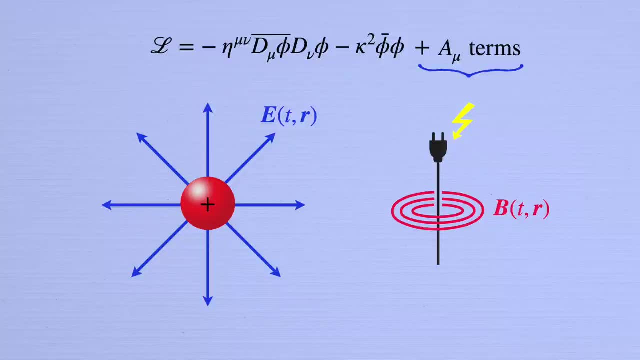 be terms for a mu in the Lagrangian- that give us Maxwell's equations when we apply the equation. So let's take a look at some of these equations and see how they work Again. I'm just going to quickly tell you the answer right now. 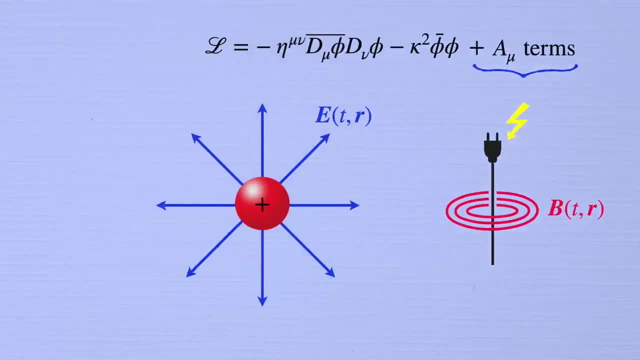 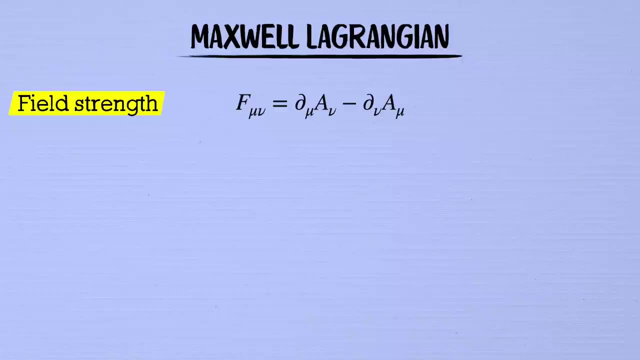 and in the future I hope to tell you more about where it comes from and what it means. From the electromagnetic potential a. we define the electromagnetic field strength by taking a couple of derivatives: f mu, nu equals d mu a nu. minus d nu a mu. It's a 4x4 matrix again. 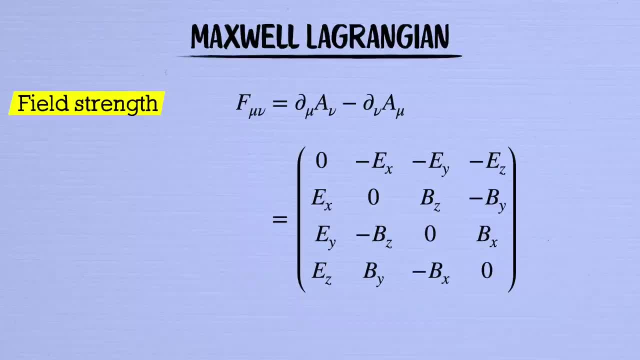 that packages up the electric and magnetic fields in a particular way, like this. But we don't really need this whole matrix right now. Using f mu nu, the Lagrangian for pure electromagnetic potential, is actually very simple. It's basically just f squared where this combination with the 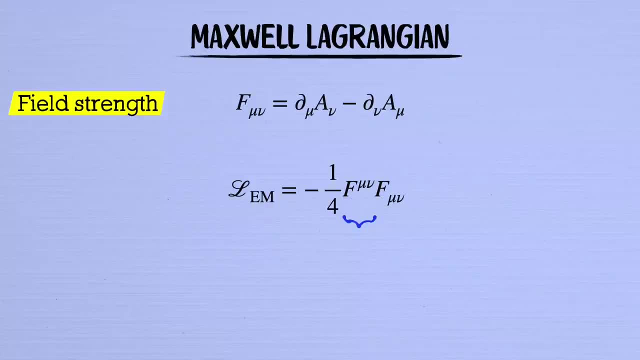 upper and lower indices is another shorthand. Sorry, there is so much notation in this subject. It's what we get by matrix multiplying with eta to raise the indices. It looks like something fancy, but again, the point is just to take care of those pesky relative minus signs between time. 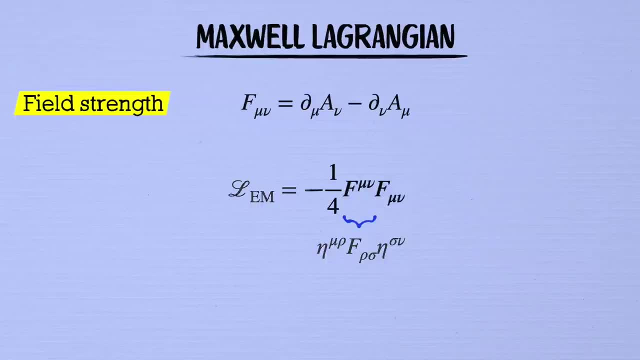 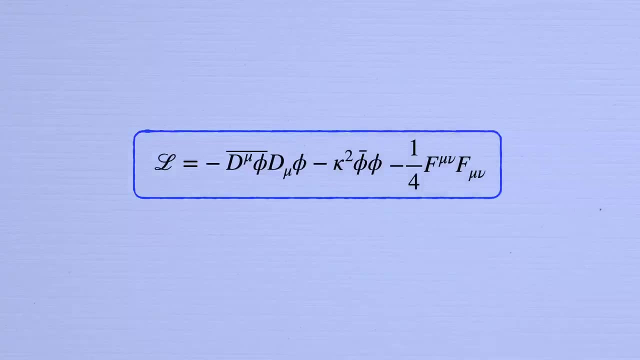 and space terms that always come up in special relativity All together. then here's the Lagrangian for the electromagnetic potential a and our electrically charged field, phi. If all this is new to you, then this is a ton of information to take in so quickly. 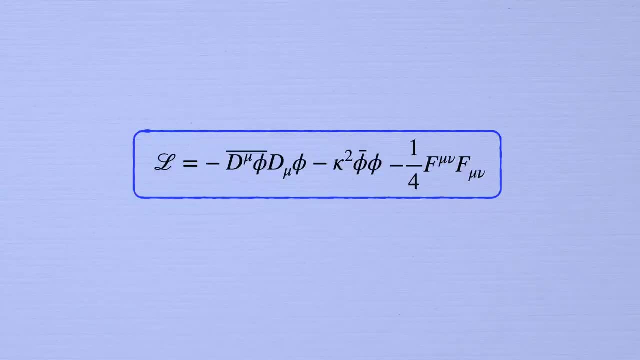 So just take this as a teaser for future lessons where we can dive into more of the details. Speaking of which, let me finish with one last teaser. What we've been talking about in this lesson, by putting the Klein-Gordon theory together with electromagnetism, is called scalar. 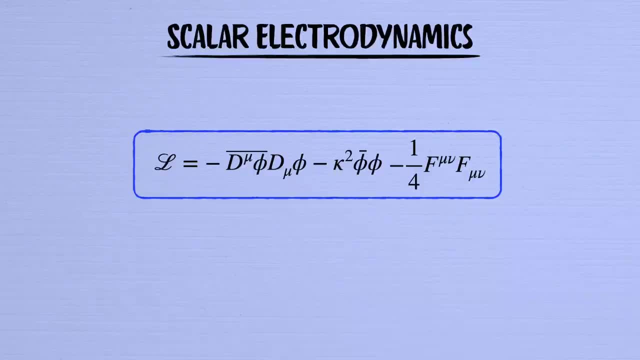 electrodynamics, And it's a good example for starting to learn the ideas of symmetries and gauge theory without too many extra technical complications. And it is physically relevant because the piece of the standard model that we're going to look at today is called the. 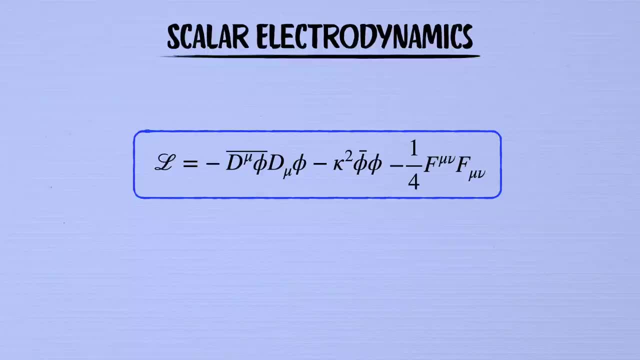 Lagrangian for the electromagnetic potential And it's a good example for starting to learn the ideas of symmetries and gauge theory without too many extra technical complications. And it is physically relevant because the piece of the standard model Lagrangian that describes the Higgs boson is a generalization of this theory. But the most 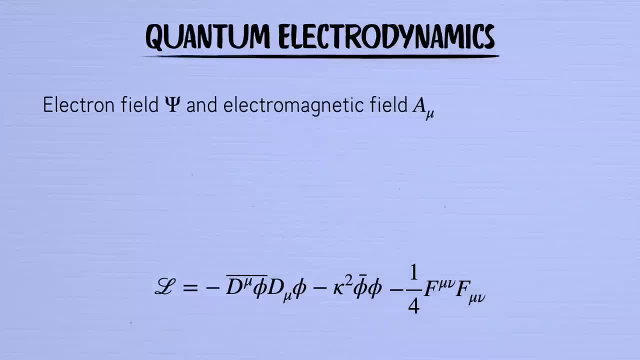 fundamental theory of electromagnetism is the theory of the electron field and the electromagnetic potential. That's called quantum electrodynamics or QED, and it was the first piece of the standard model of particle physics to be understood. The electron is not described by a scalar field like 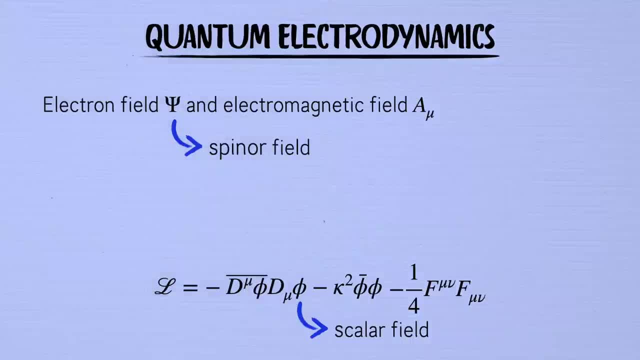 phi It's called a spinner field, usually denoted as psi. Here's what its Lagrangian looks like. Spinners make things a little bit more mathematically complicated, but the ideas we've learned here go over directly to QED. It starts with the theory of a free electron.